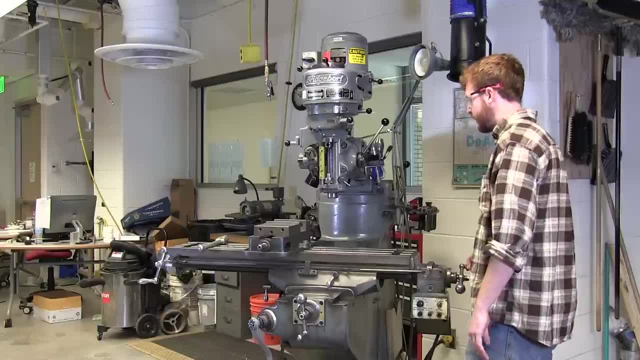 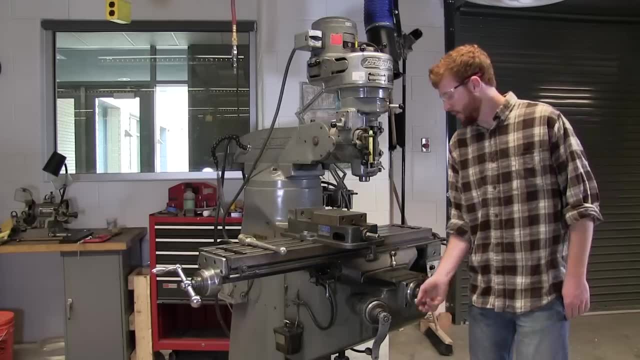 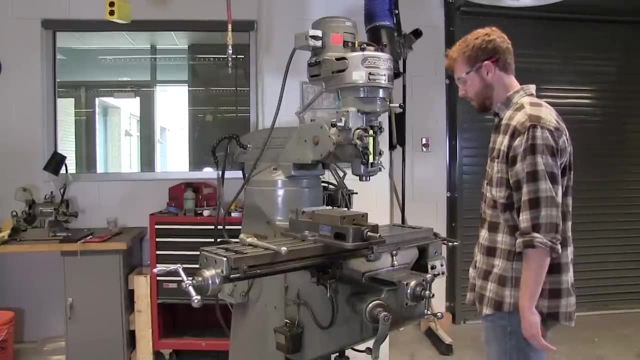 moves the table left and right and counterclockwise moves the table towards you and clockwise moves it away from you. This handle moves the table forwards and backwards relative to the operator, which stands pretty much right here. It also has a Z-axis which raises. 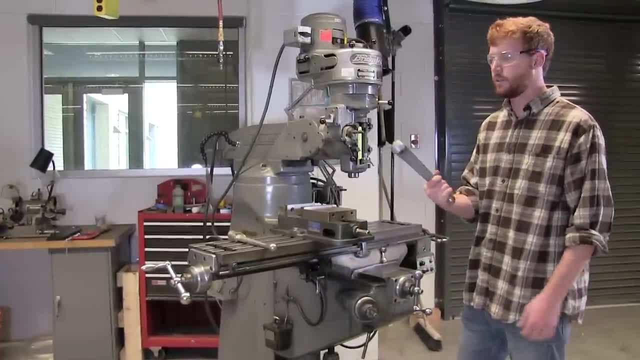 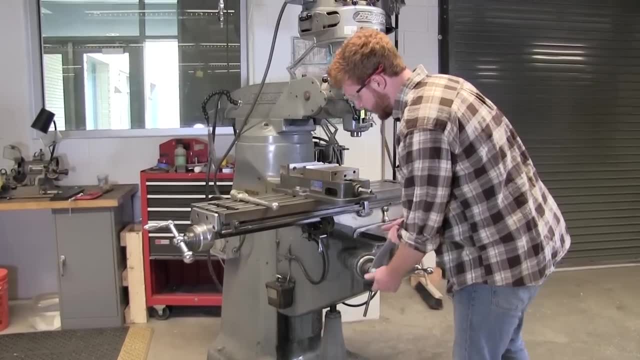 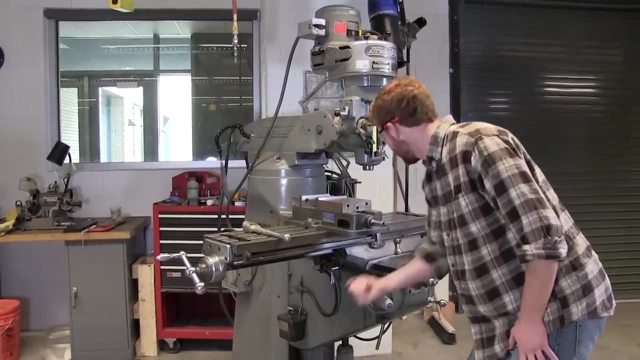 and lowers the table. This is the joint, the knee joint, which attaches to that axis, like so, and the up direction is marked on here, So clockwise- raises the table like so, And when I'm done using this, if it's going to get in my way, I'm going to be using this. 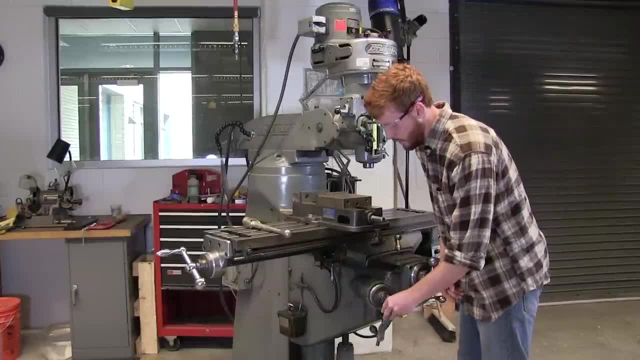 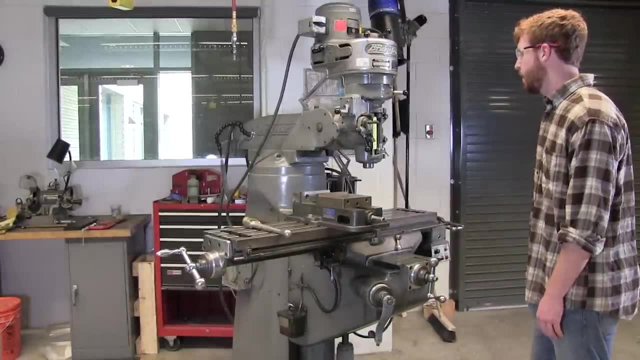 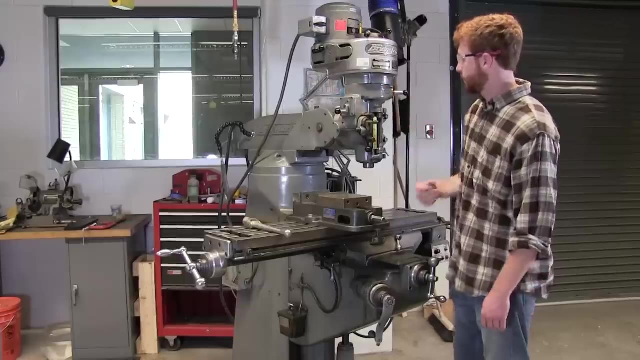 tool. I like to flip it around and put it on like so, so I can't kick it or mess with it, So I have a good, clean cut. Moving on to other operations, the on and off switch is right here. There is currently nothing in this bit in the chuck We can put any type 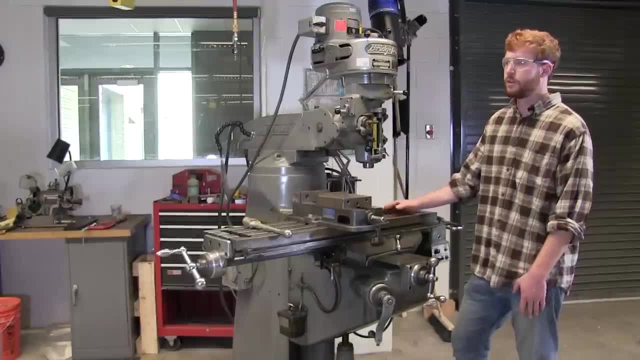 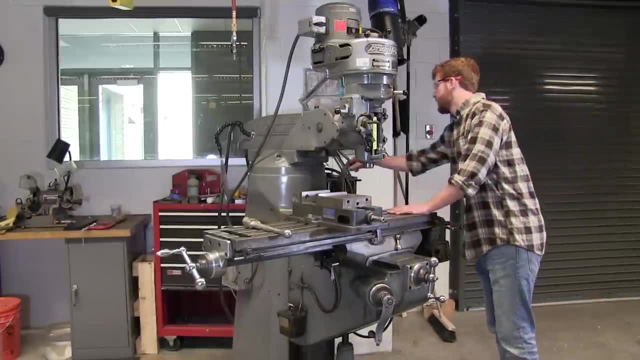 of tool into this machine that will fit into the collets. So I'm going to go ahead and show you how to do that. I'm going to show you how to load one of those into the machine I'm going to be loading. 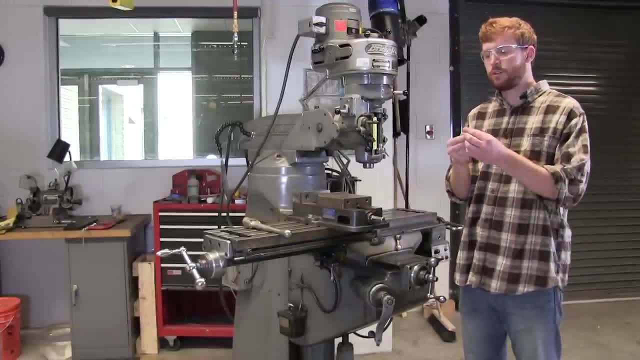 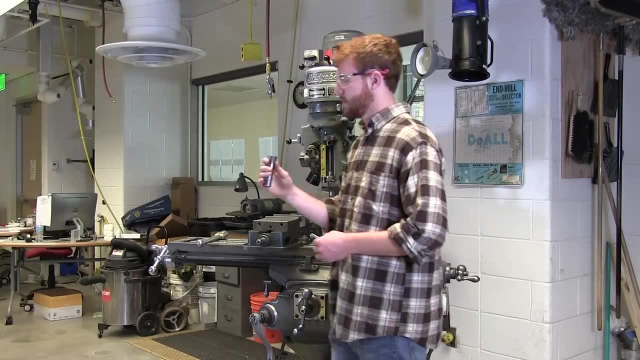 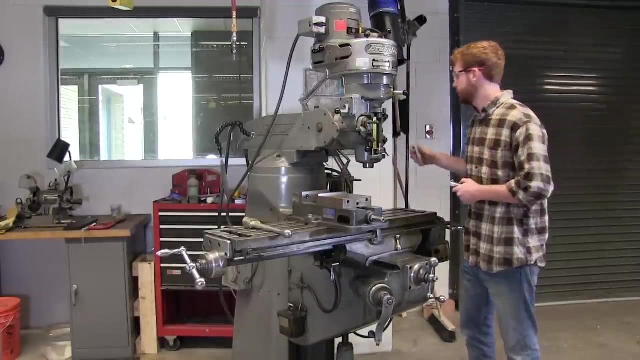 this edge finder to show how to find the very edge of a part or zeroing it. We have these collets. like I said, Each one has a different diameter. We have big, small. Each of them should be marked with the correct size that it is. 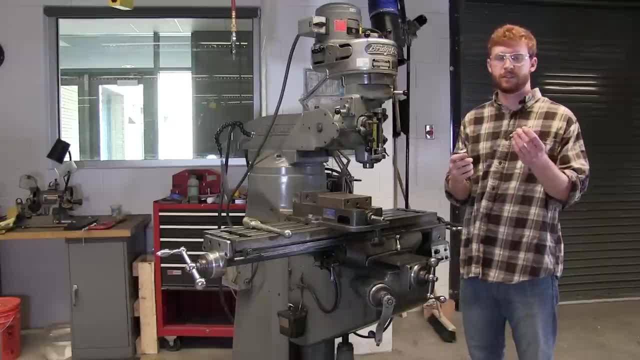 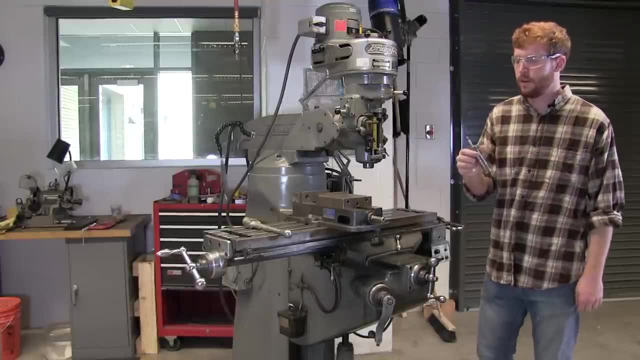 This is a three-sixteenths inch collet and this is my three-sixteenths inch edge finder, So I'll put it in like: so It should be a press fit pretty snug already. And then what happens is there's. 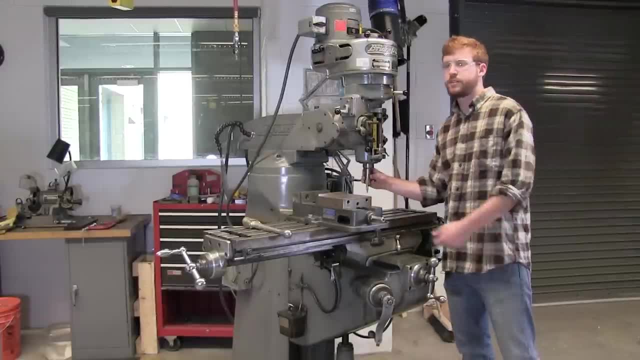 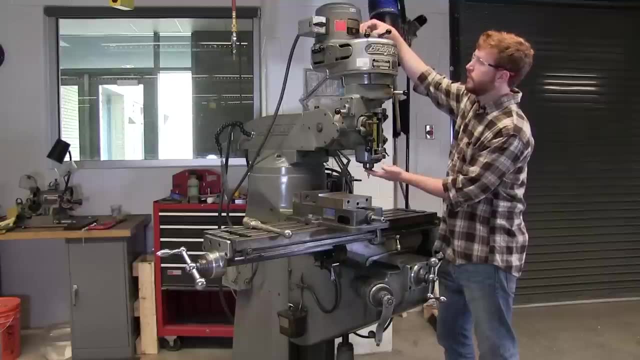 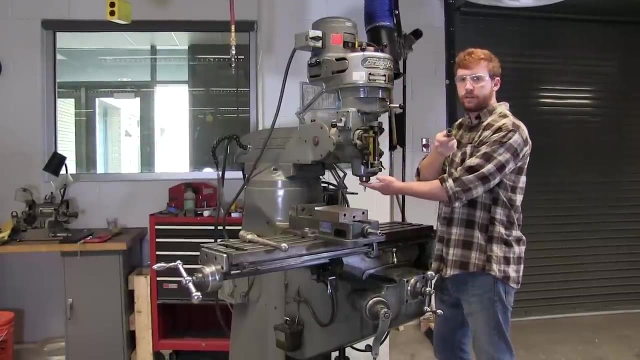 a keyway on these collets, which finds a key in the chuck. I'll go ahead and press the collet all the way up against the machine and this shaft right here screws into the threads which are on the back of these collets. 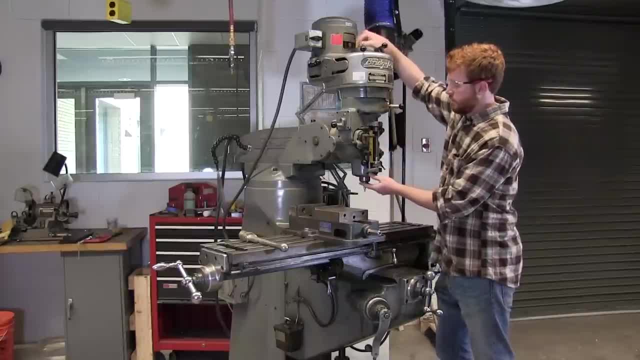 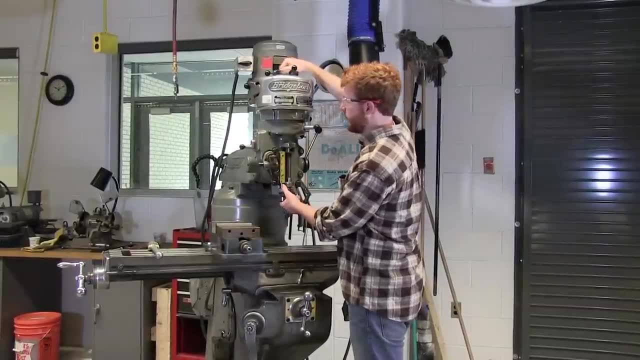 So I'll hand-tighten that first, with my hand kept on the collet, to make sure that it doesn't fall out, so it doesn't damage the bit, or maybe if I had a part in there it would damage the part. 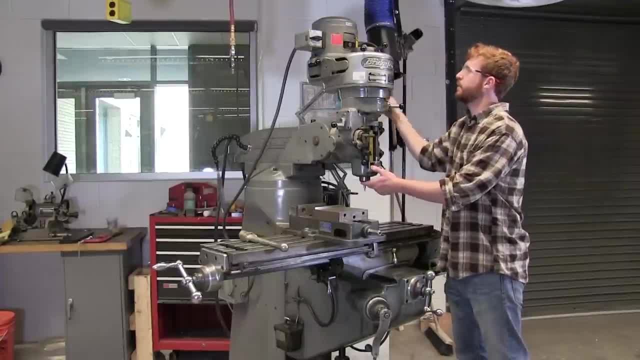 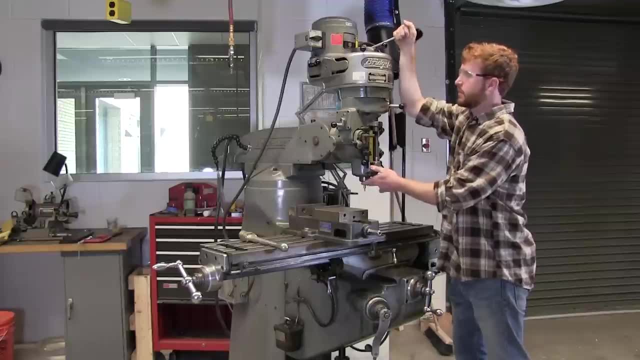 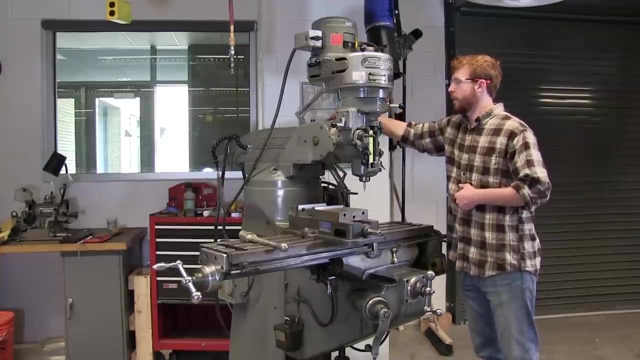 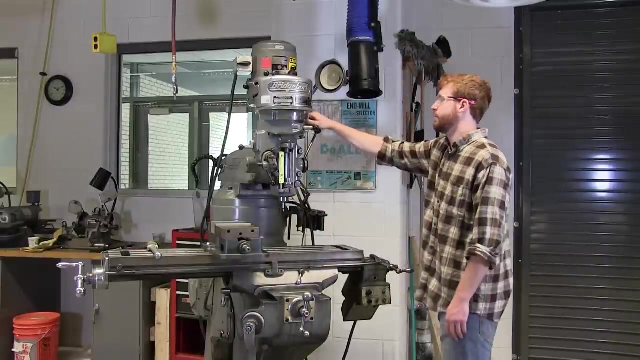 I can grab this wrench which is back here tightening. Try to get it nice and snug. get in some taps, but not too tight that you can't take it out again if you need to Put that back. Right now the machine has a brake on which is on this side over here There's. 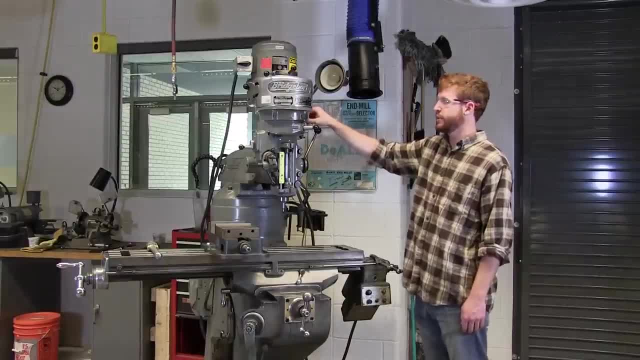 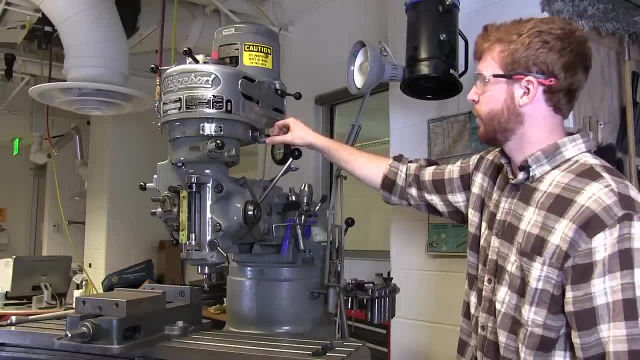 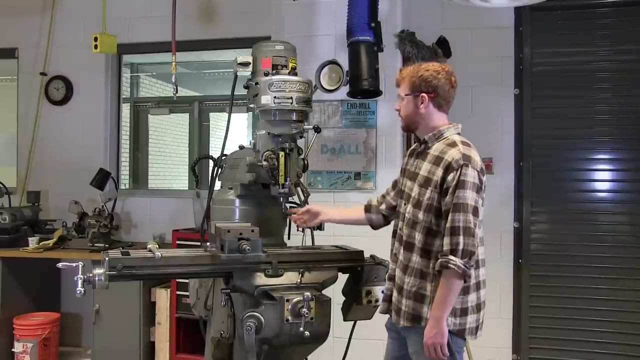 an in position and an out position. The in position means the brake is on, meaning that I can't turn this. So I'll move the lever to out by pulling out this black pin. and now this machine is free to move. So to use this, I'm going to be putting in a part into 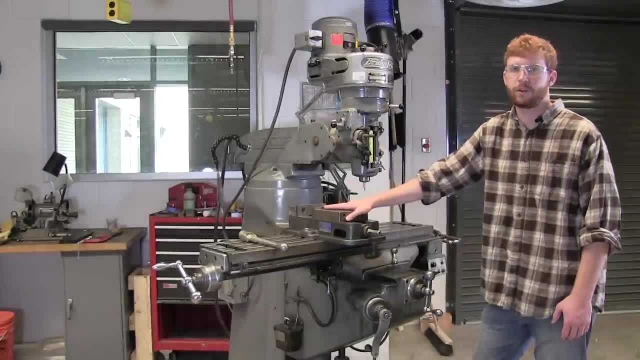 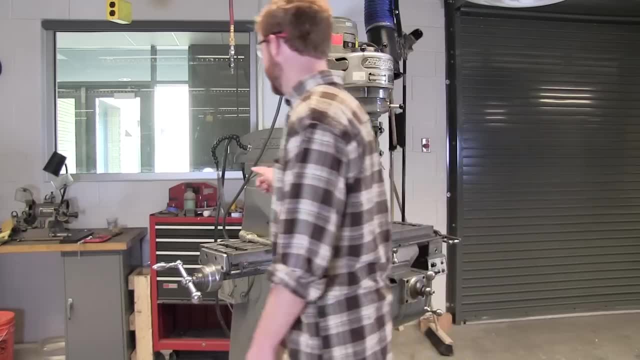 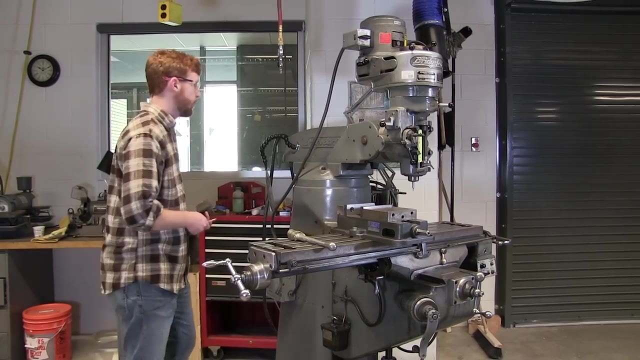 my vise. So this is the vise which holds anything that I'll be working on, anything I need to be holding while I'm cutting it with this tool. So over here I've prepared what I need to clamp my part into the vise. This is the material that we'll be working with. 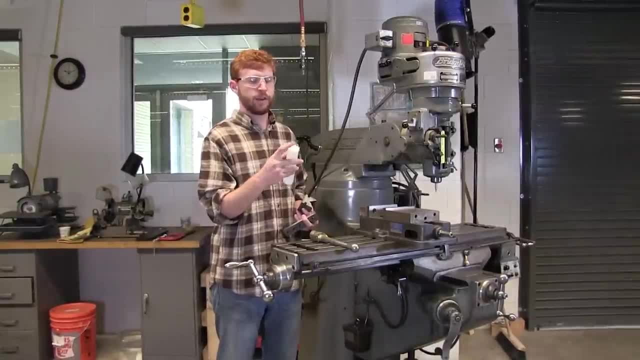 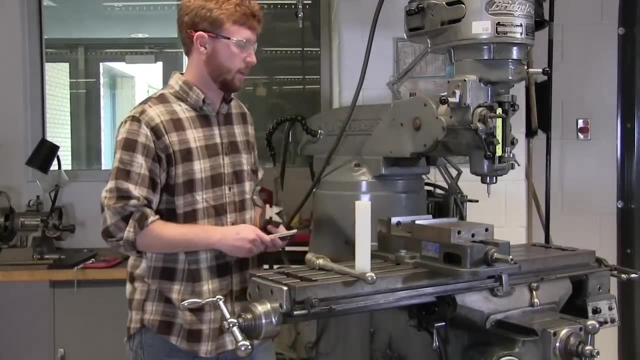 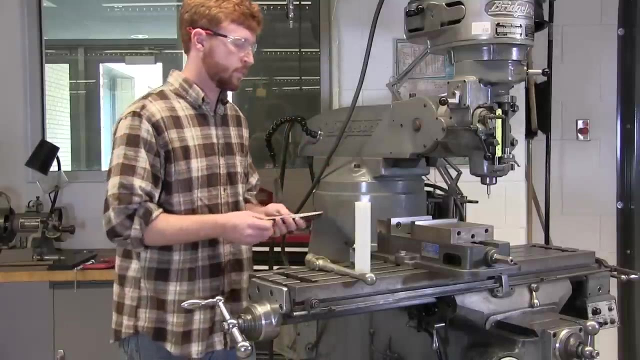 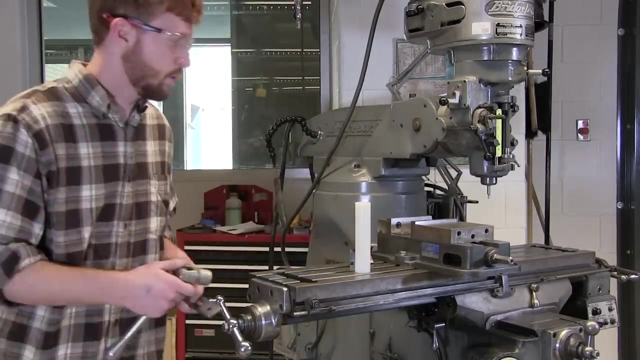 today. high-density polyethylene. I went ahead and faced this side, so it's nice and smooth, so that this edge fits. So I'm going to go ahead and make a cut. I'm using these parallels. They come in pairs, totally parallel, hence the name. I'll be using them as spacers for these grips today. 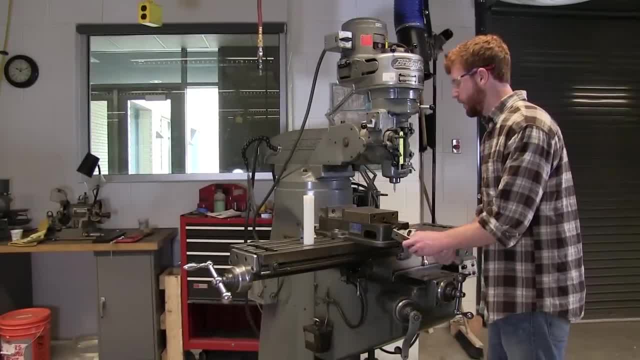 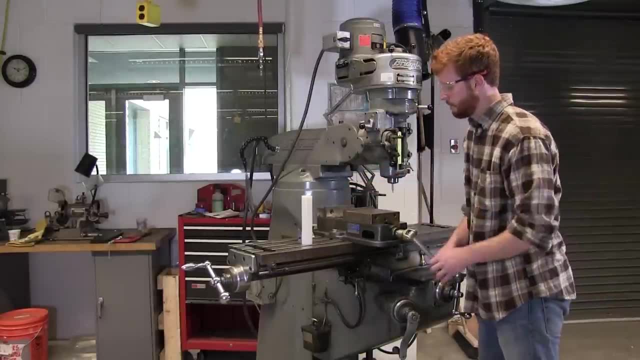 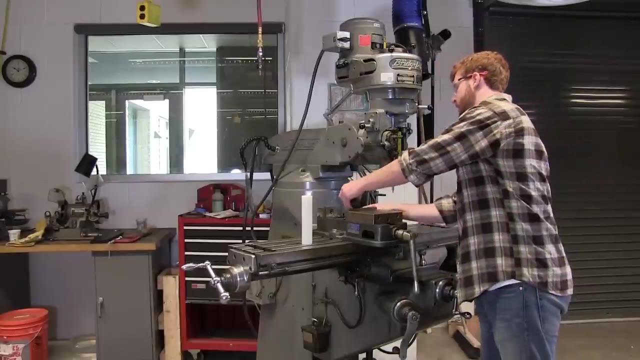 So with this I can open and close the vise. So open it, put my parallels in, try to make sure that they look nice and straight, Jump my little grips in there and then I can go ahead and put in my part. 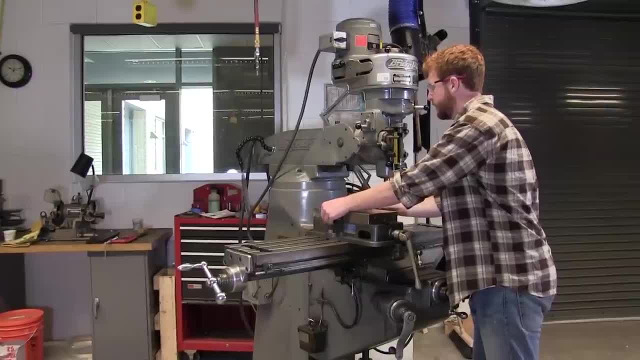 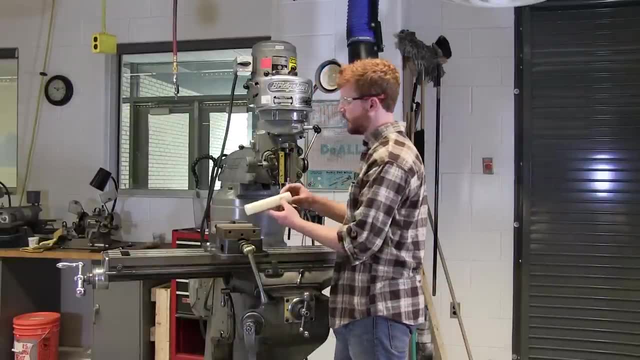 When setting in my stock part that I'm using. I'm going to go ahead and put this in, so it's like hanging out a couple inches. I'm actually going to be facing this side of the vise, So pretty much perfectly right here. 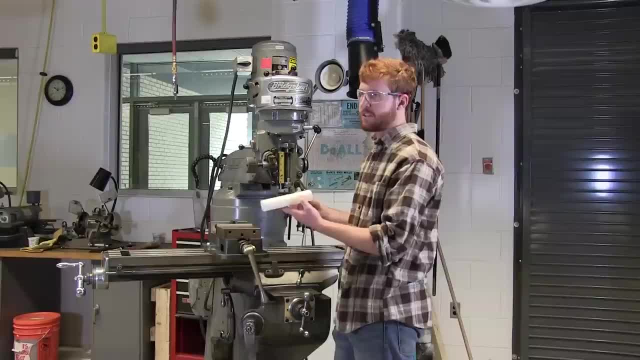 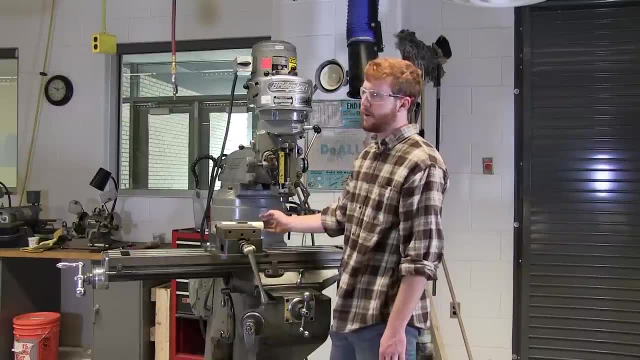 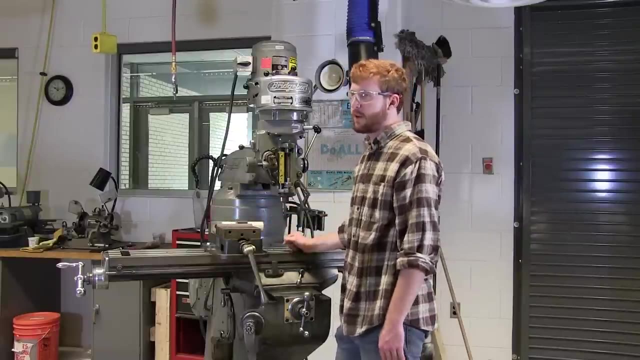 it about an inch deep, just as an example cut. so I'll put this in there, leaving whatever I'm going to be cutting, the area I'll be cutting hanging out of the vise so that I definitely won't run into the vise with my tool, which would damage the vise and damage the tool, and then I want that to. 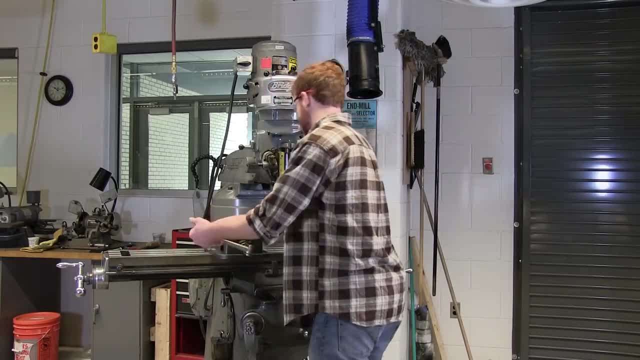 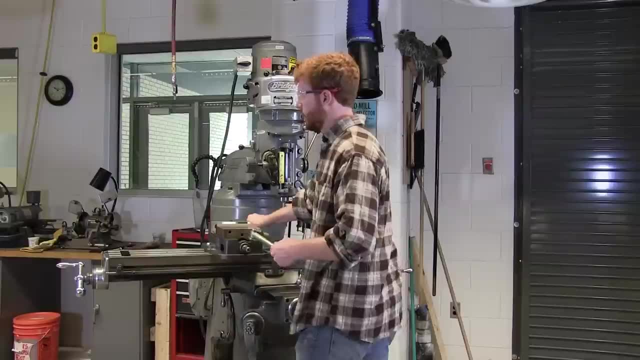 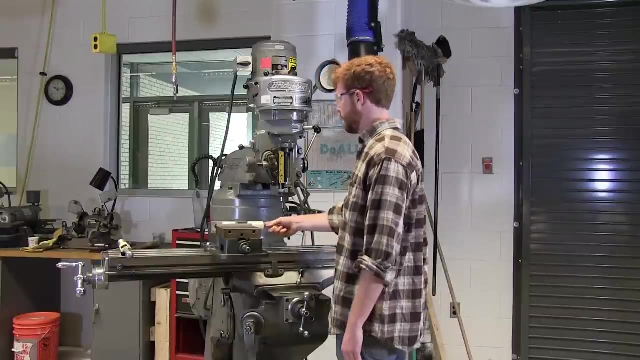 happen. so go ahead and tighten that in there same thing. nice and tight. this material is kind of soft, so I'm not going to really crank it in there, but just so that it won't move and I can go ahead and turn on this edge finder and find that edge. so the on switch is up here. I'm using the. 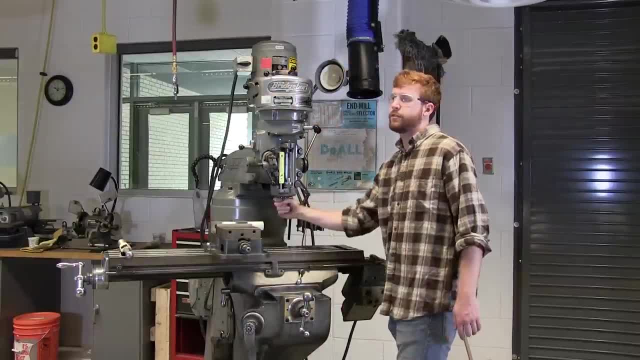 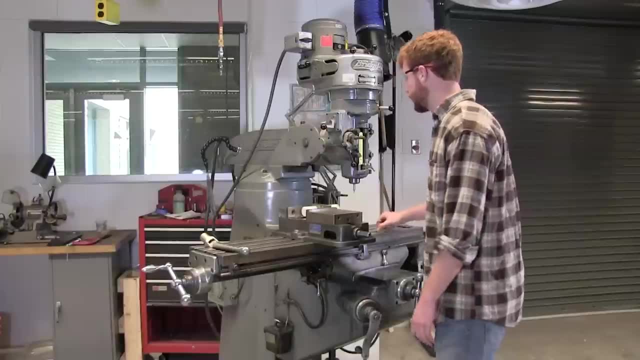 forward direction. I'll double check, make sure my brake is off. that would make a horrible screeching noise if I were to leave that on. so I'll leave that off, go ahead and turn this on and basically just butt this up against the side of this face. 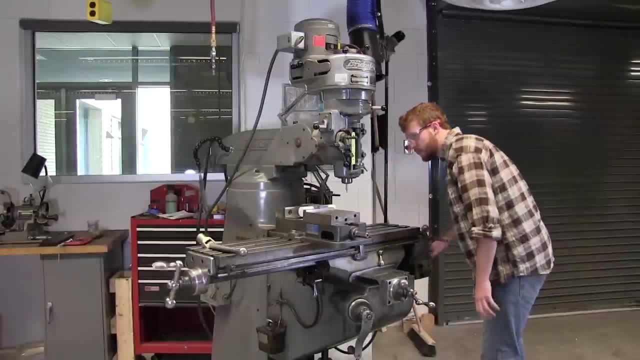 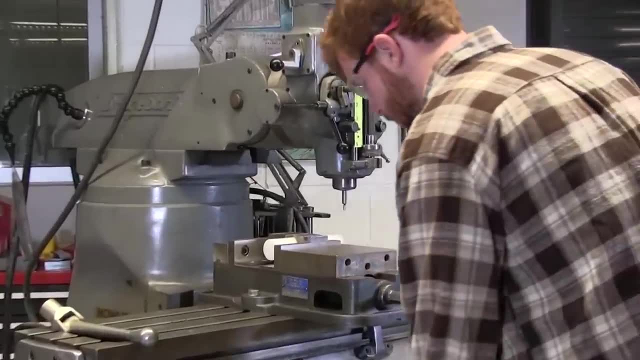 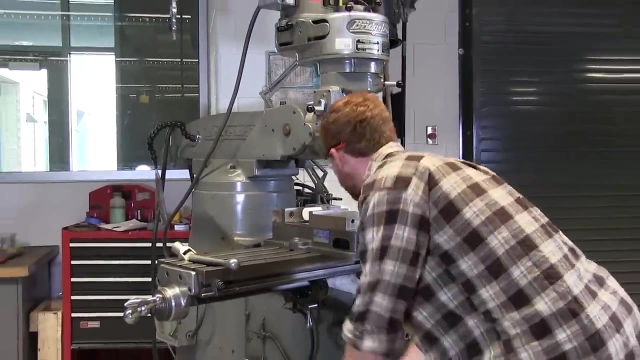 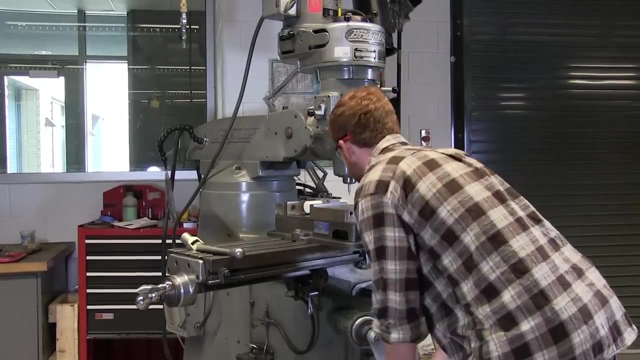 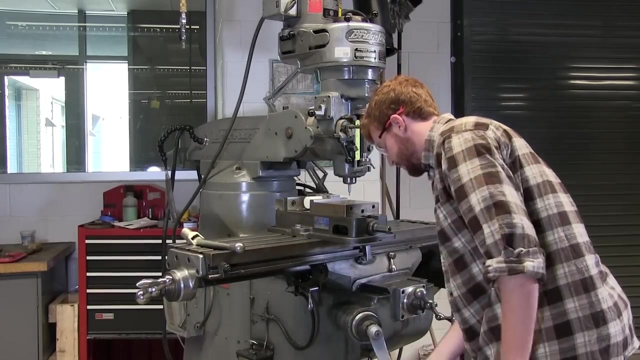 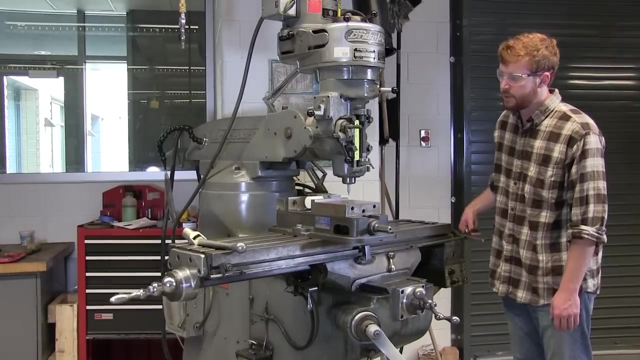 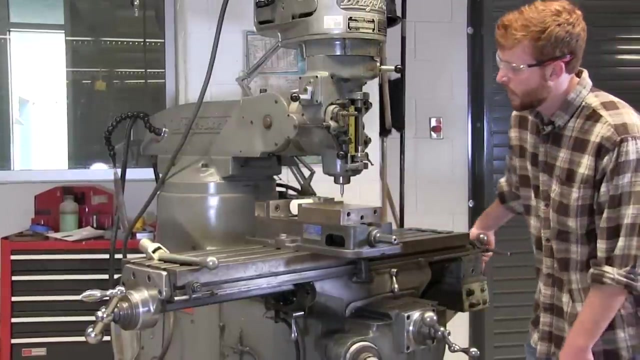 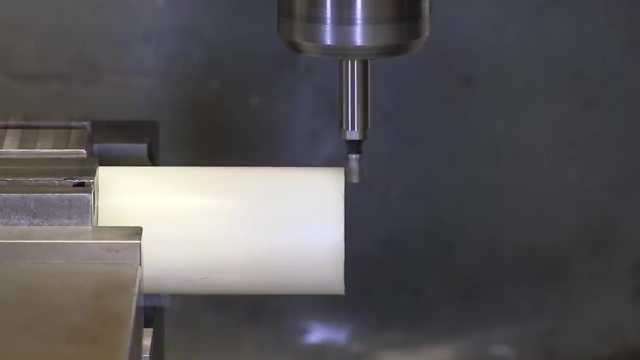 so. so I'll bring the part up against my edge finder and I'll watch it. it has a movable end at the bottom, and as I bring it up and butt it up against that face, it'll slow down its shimmying until it's pretty much perfectly centered, and then I know it's centered once, the center actually. 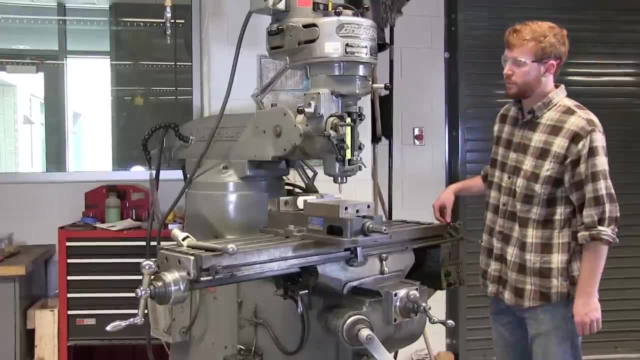 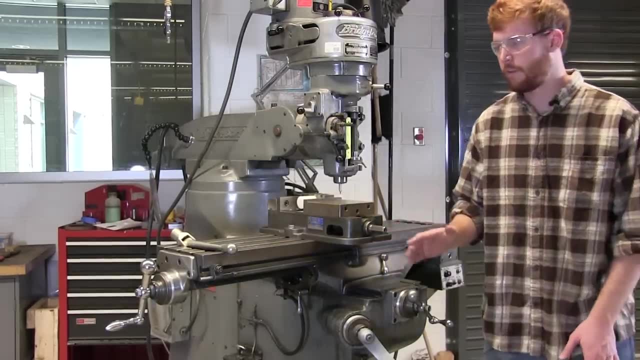 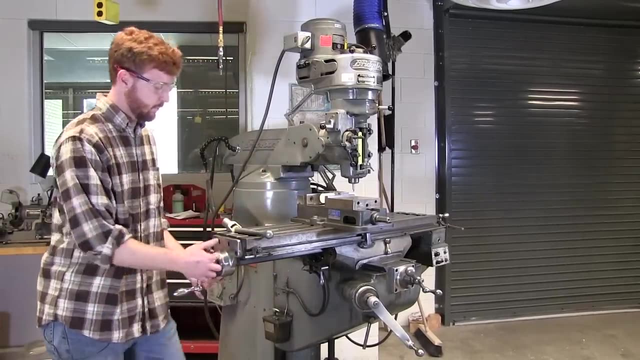 breaks off like so. so you'll see that the edge finding bottom has actually moved away from the center. that's how I know that I'm right on that edge, so I'm going to zero that point. each of these dials has different indicator scale. as to your position, it's in thousandths of an inch, so each 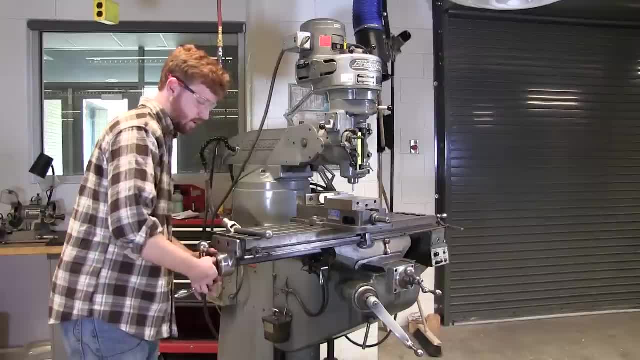 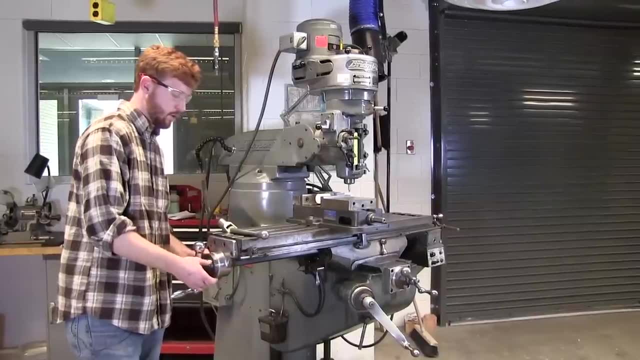 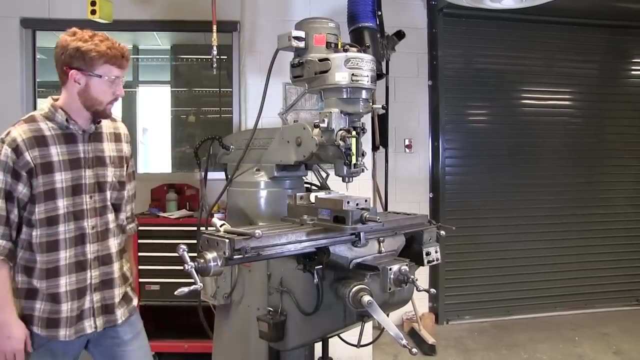 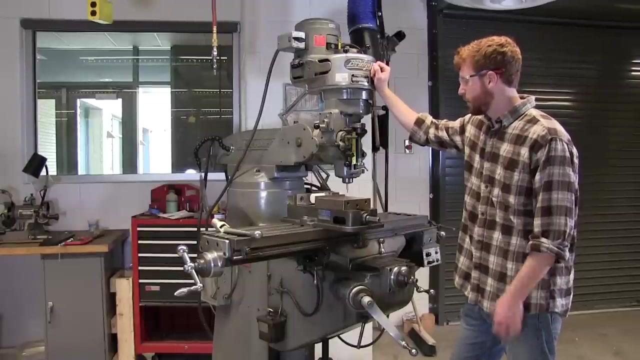 tick mark is one thousandth of an inch. I'll loosen that up, set that point so I know where that is. again I can find it again, move it away, turn it off. so now that I've found that zero, I want to check it again and make sure that I actually have that. 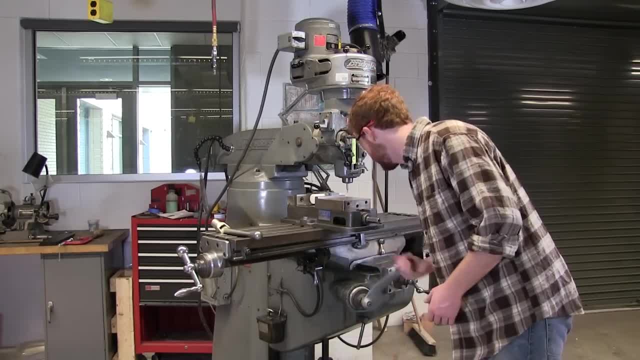 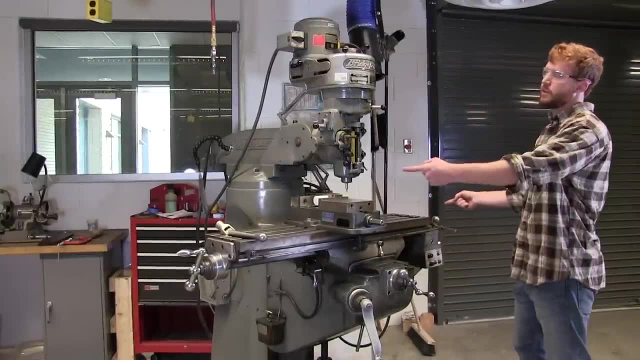 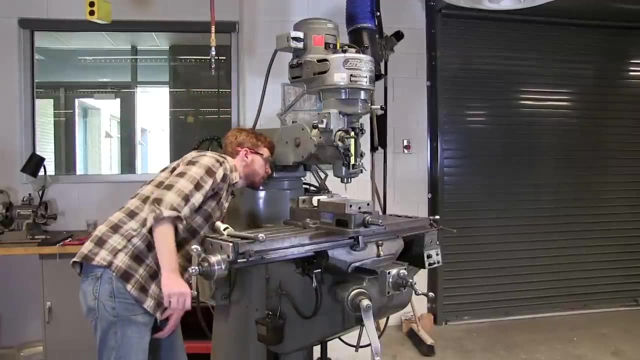 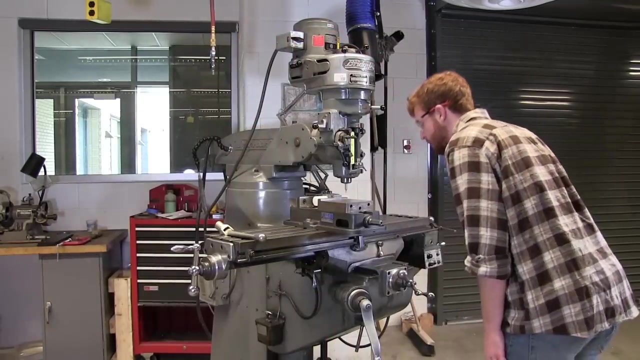 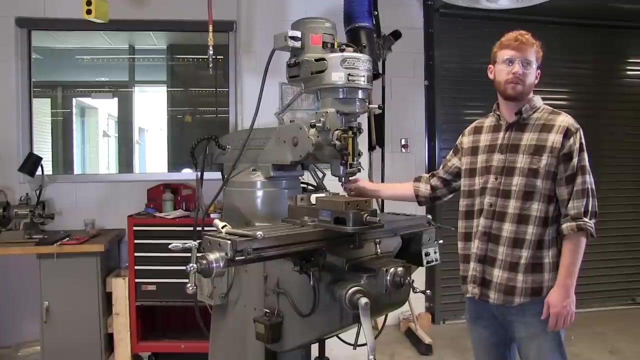 at that zero point, so I'll lower the table and move this over. both of these sides of the table have dials, but I use this one, so I'll go up to this guy and bring that to my zero point, which is right there. so what I found is the exact center of any tool that I'll 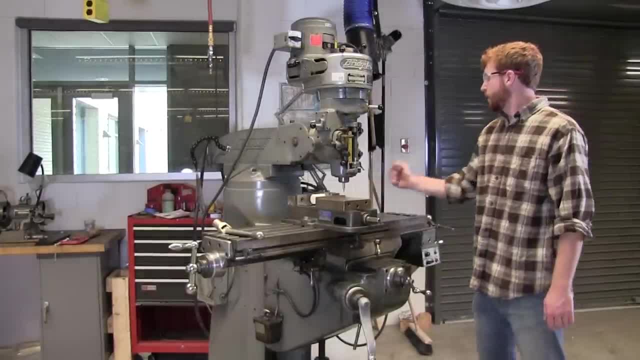 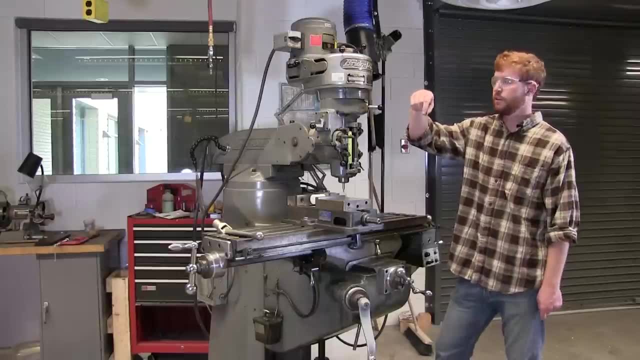 be putting in here, so I can go ahead, change this one out for the tool that I'll be cutting with, and then I'll be able to go to the next one and see how much I can cut with it, and then you can to make my cut, which will be a depth of one inch into the part, and cutting down about. 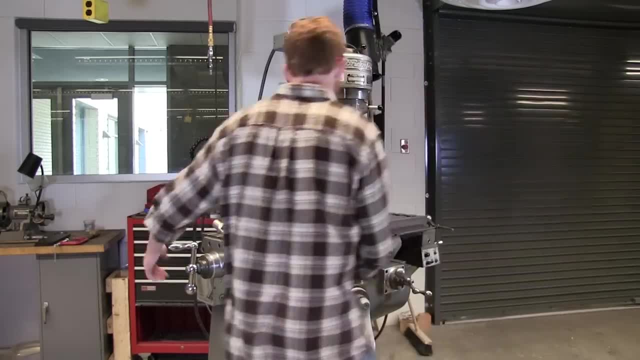 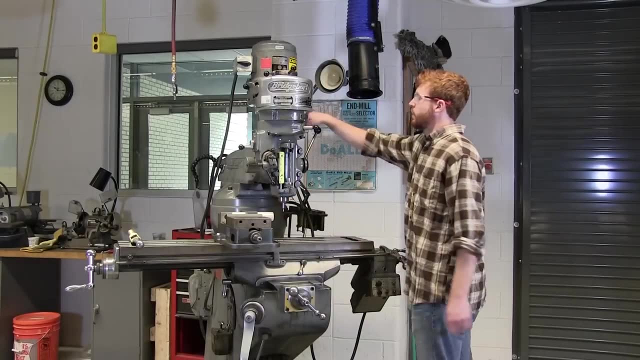 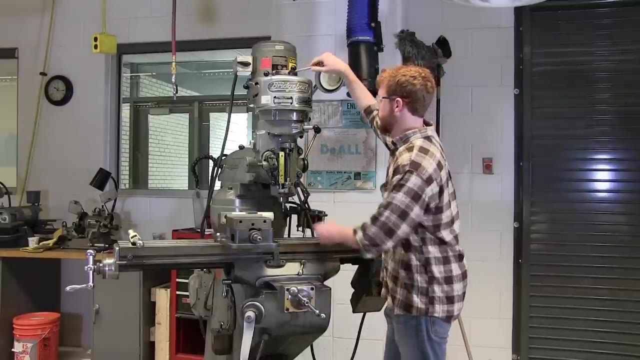 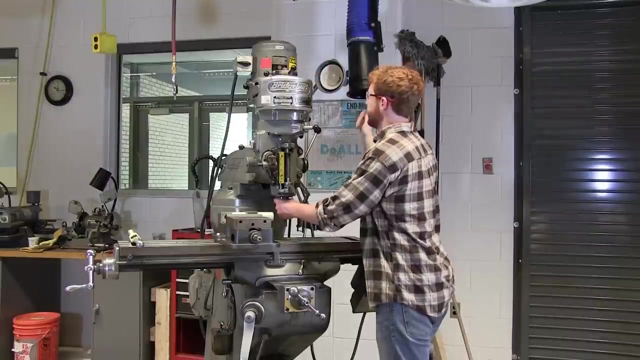 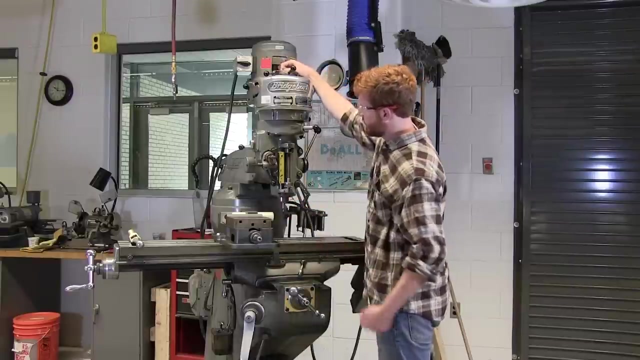 a quarter of an inch, So I'll move this away. I'll make sure the brake is on, which makes loosening the bit much easier. Put this back undo it if the collet gets stuck in there. I'll actually keep this threaded. 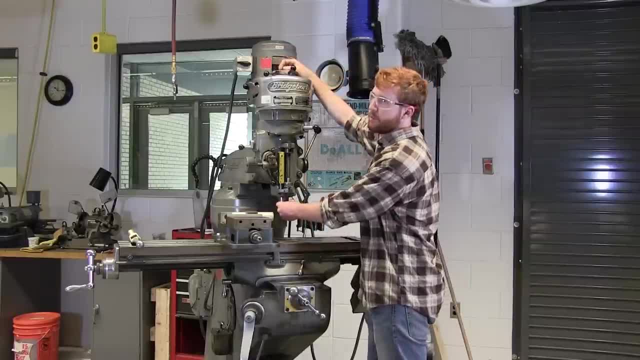 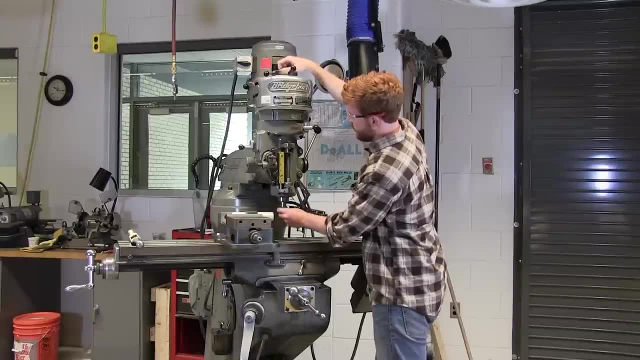 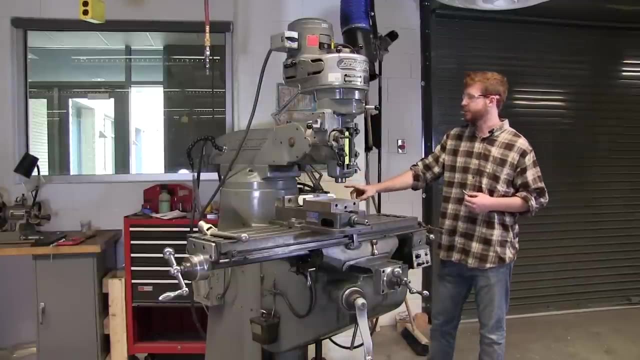 and actually give it a little bit of a tap which knocks it out of place without damaging the threads too much. So I'll unscrew this the rest of the way. Okay, Take this out, put these back where I found them. On this mill there's a nice holder for all the collets and they each have a space. so 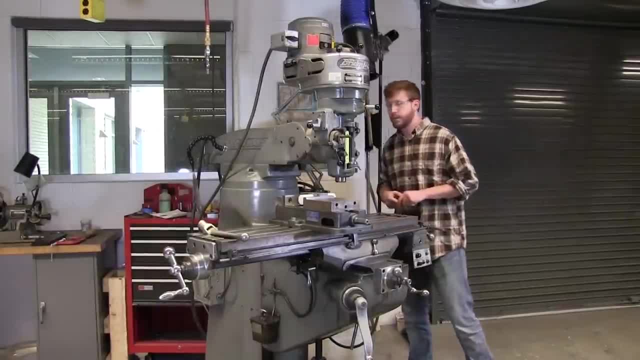 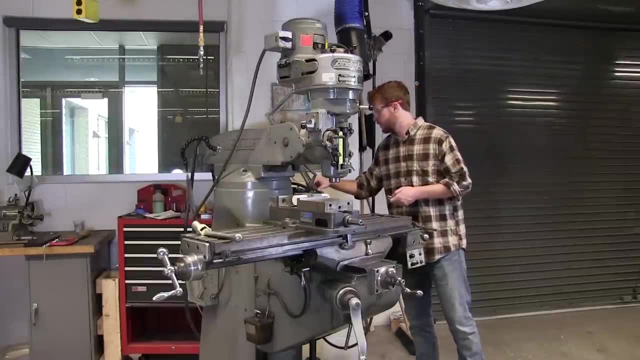 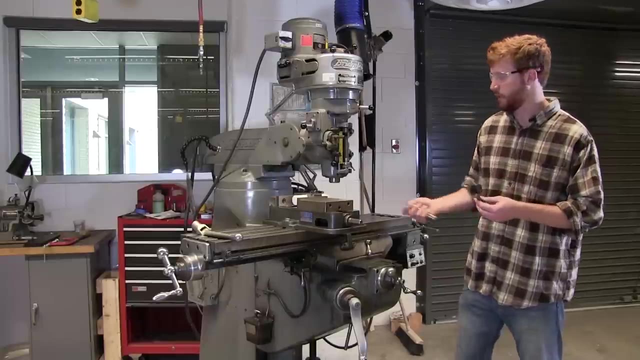 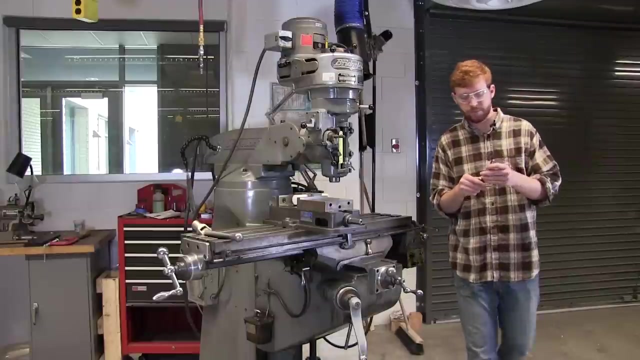 make sure that they go back to where you found them. For the cut, I'll be using a half inch end mill. This particular tool has two flutes, which is suitable for cutting this soft material. If it were steel or aluminum, You might want to think about having more flutes, but you can learn about that and feed. 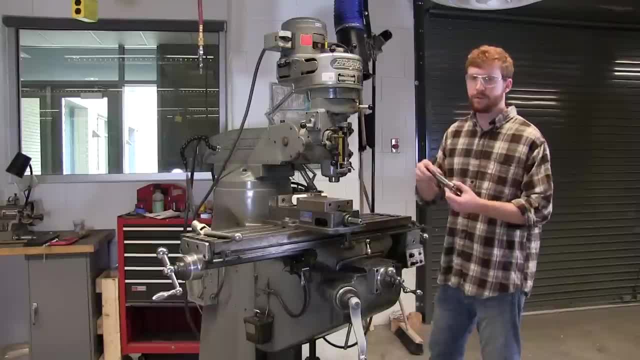 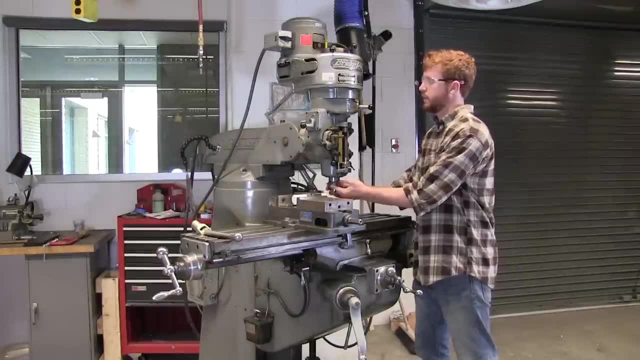 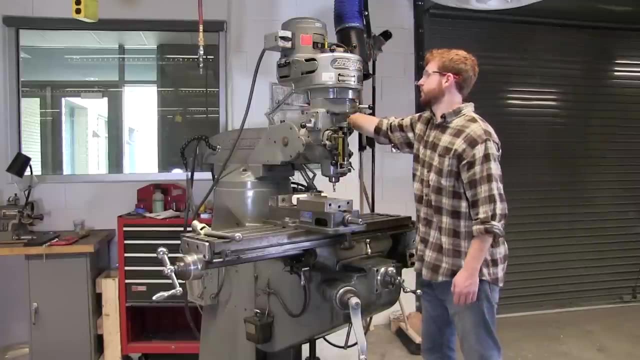 these beads and manufacturing processes Same thing. there's a keyway. I'll line it up with my key Inside. just spin it around and there we go. Push it up, Tighten this all the way down, Not too tight, Okay. 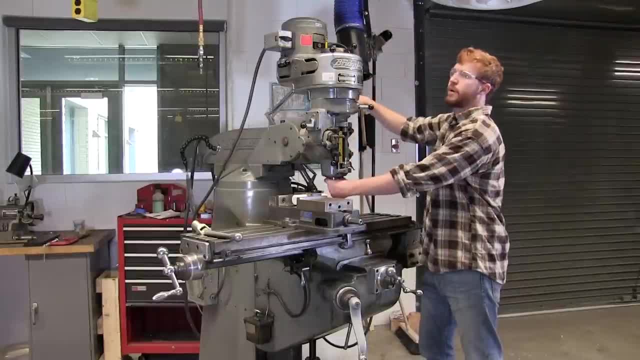 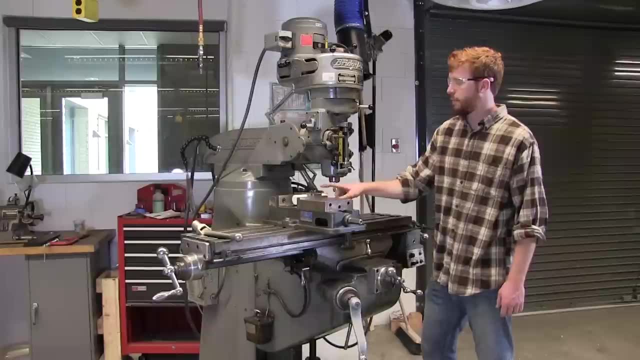 There we go, There we go, There we go. Make sure my brake comes off. so this is free spinning and I'm good to go. So now I have to find the very top of this part so that I can know exactly how deep I'm. 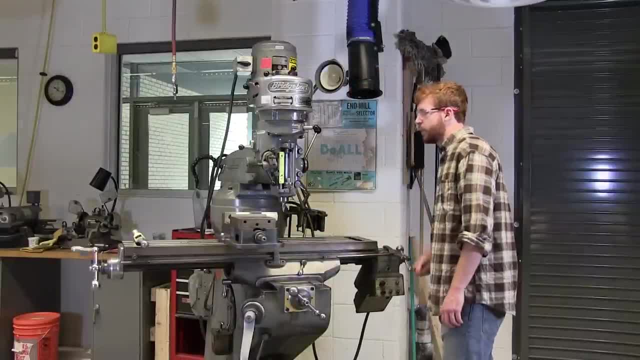 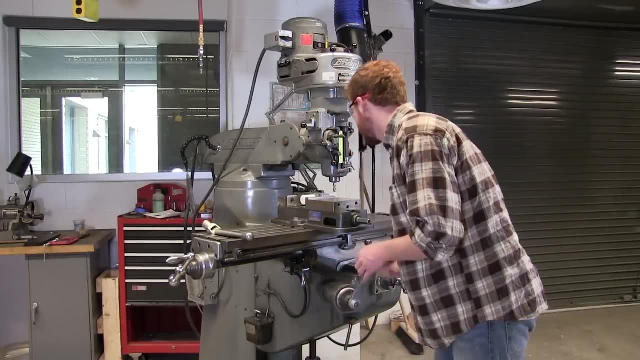 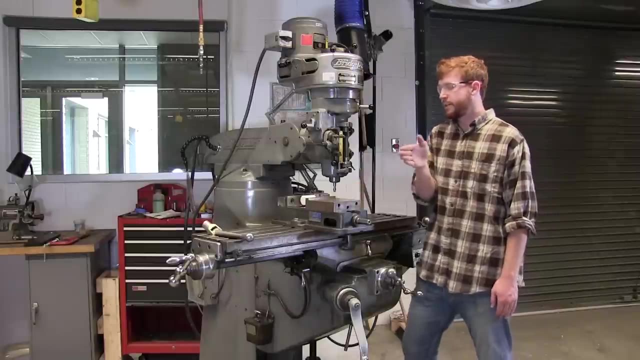 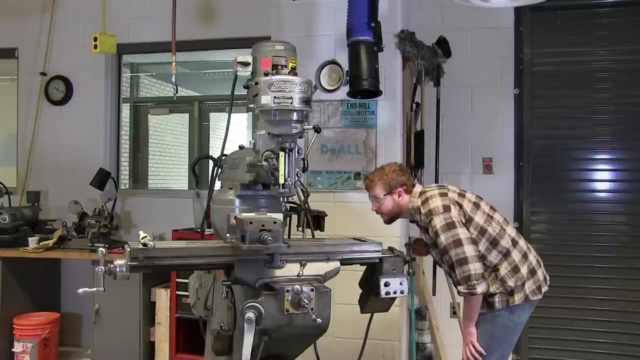 going to go. So the way I'm going to do that is, I'll line up the bit with the very center of my part. This can be found using the edge finder as well to find the outer radius And then move that distance to the very center, or you can kind of just see it with your eyes. 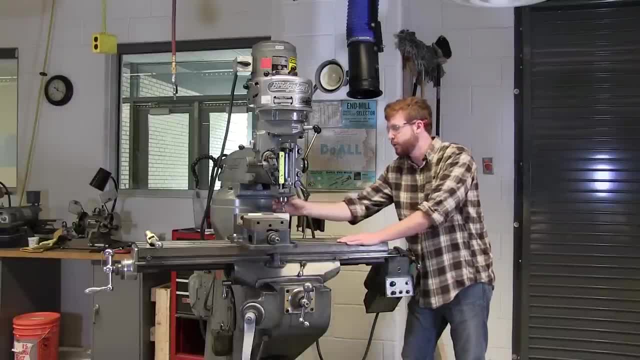 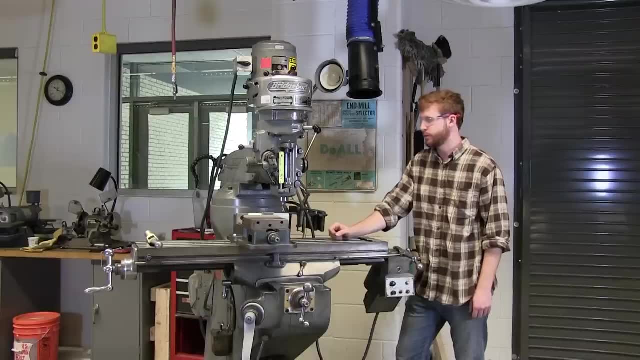 So I'm lining it up, I'm also spinning the tool and the bit so that those two flutes that I was talking about line up with the center line of this material. That's because those two flutes at the very bottom, that's where, like the deepest part, 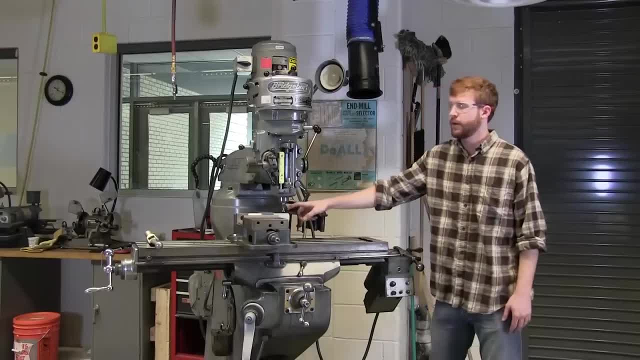 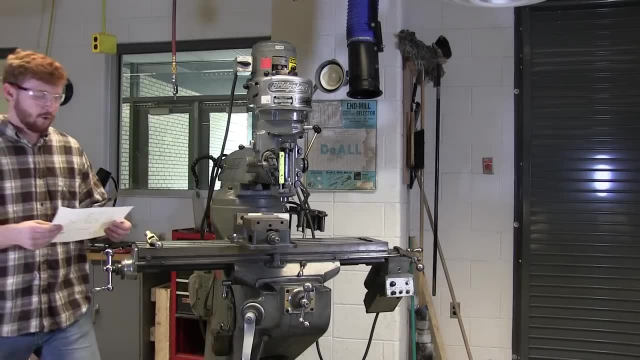 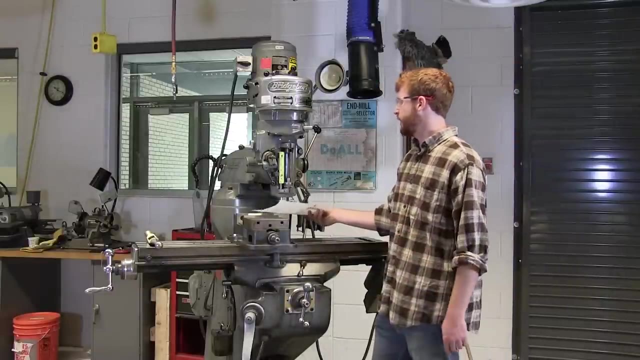 of the tool is- and that's what I want- to zero against the top of this. So I get this sheet of paper which I know is about 3 thousandths of an inch, or .003 inches, and I'm going to put that between the tool and the part. 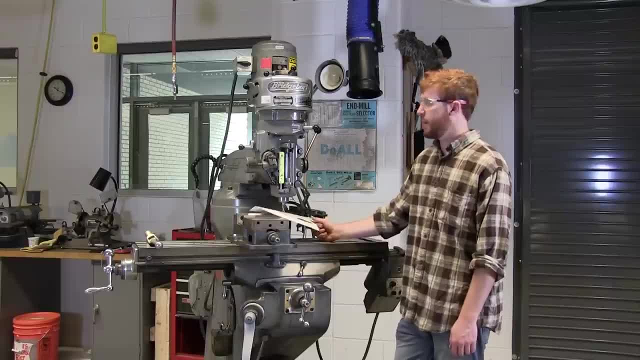 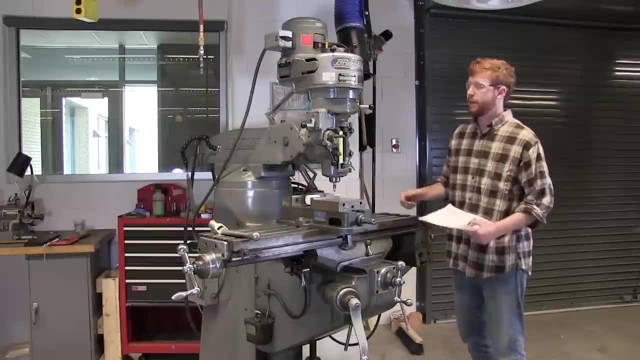 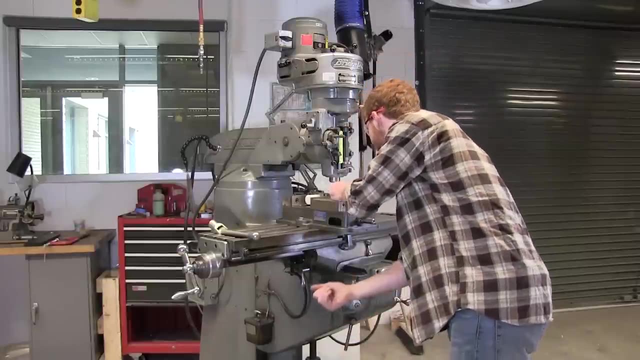 This serves to kind of have a physical barrier so I don't scratch my part or anything like that, and it works pretty well for zeroing stuff like this. So double check that I'm at the zero point, Put my paper between the tool and the part and raise my part, basically, and I'll be shaking. 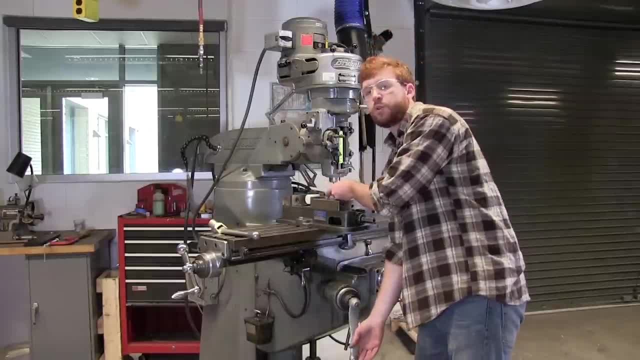 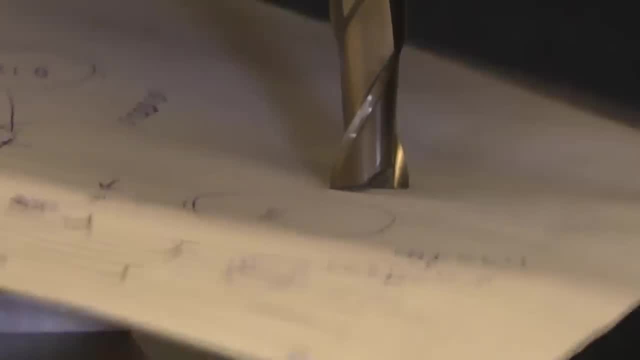 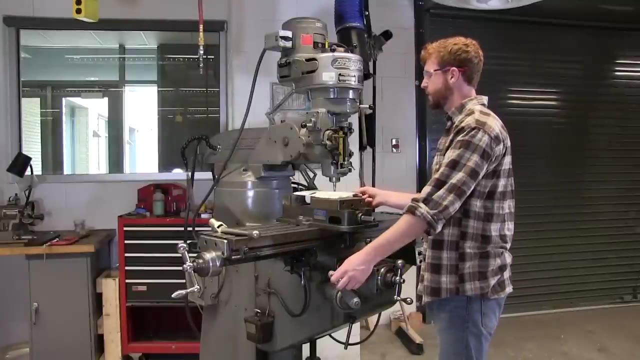 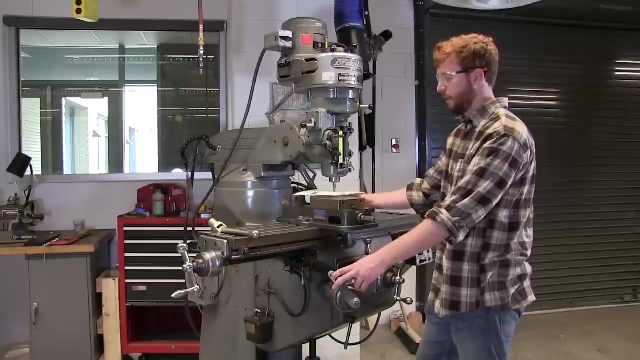 this a little bit until the tool grabs the paper. So right there. If I were to move that any more, I would actually be ripping the paper and I don't want to do that. So that's how I know that the tool is right on top of the part. 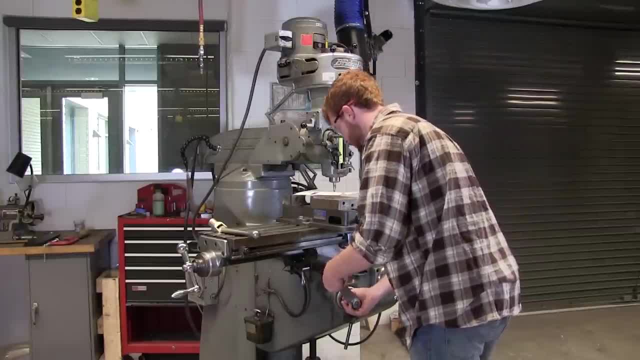 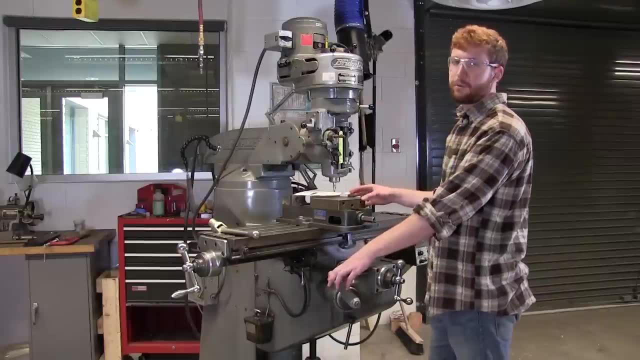 So, on this knob, I'm going to go ahead, unscrew the handle, move this to zero and remember we have a thickness of 3 thousandths of an inch of this piece of paper, So I'm actually going to offset that from my zero. 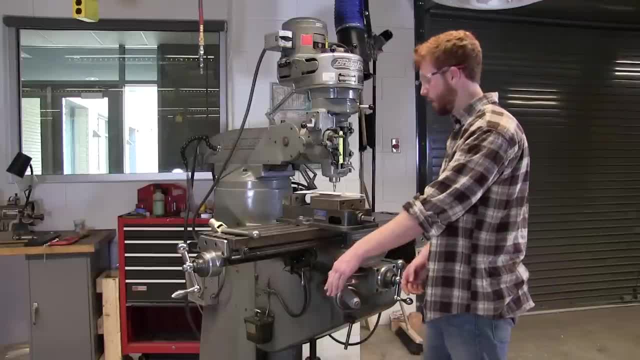 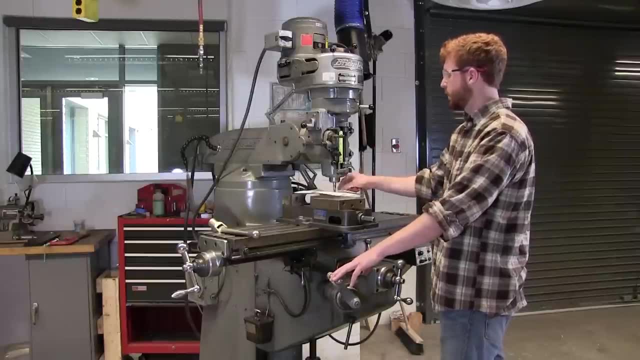 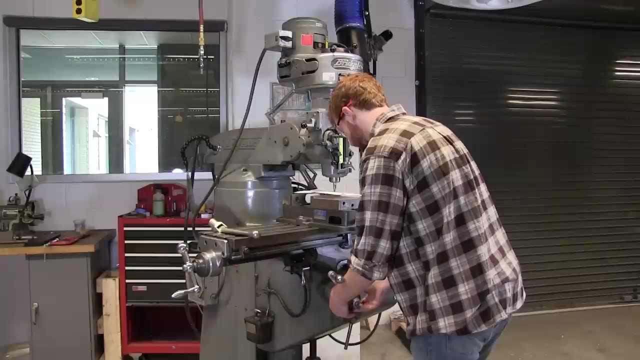 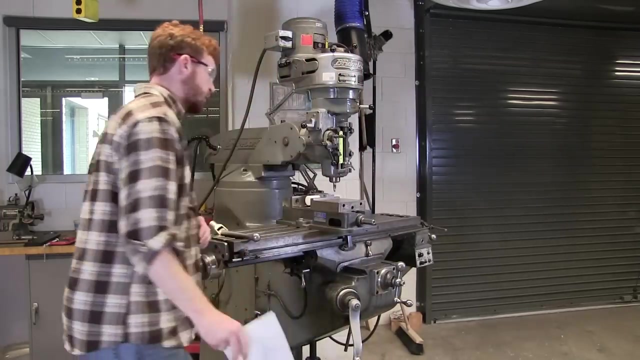 So I'll set it to about like a negative 3, if you can kind of think about it, So that when I bring this handle up those 3 thousandths, this tool is exactly on the very top of my part. So I'll go ahead and tighten that and then I'll lower my part down. 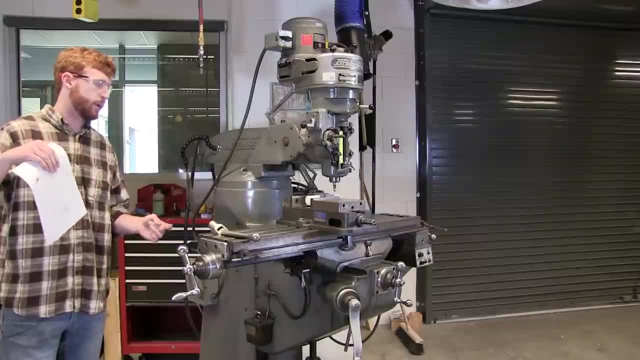 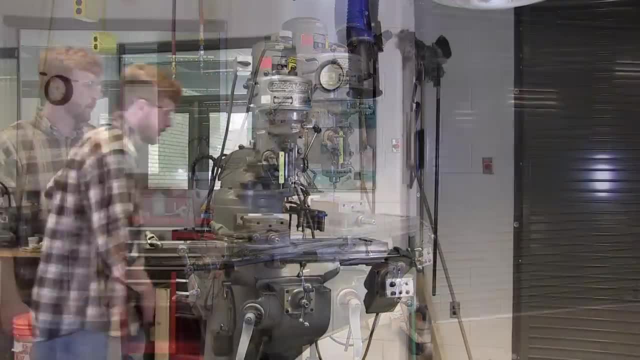 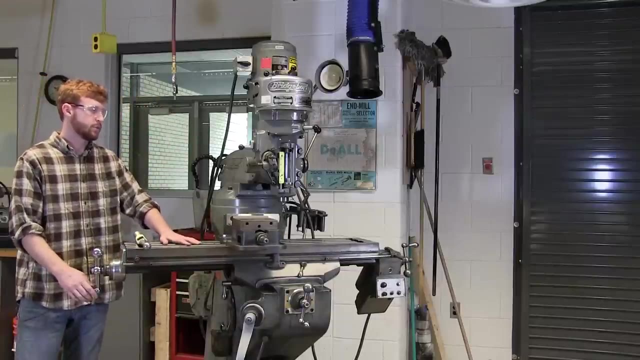 So, just like I did with the edge finder, I'm going to bring everything to my zero point. make sure that looks good to me, and then I can make my cut. So I'll take this to my zero. Another important thing about using these machines for precision machining: each of 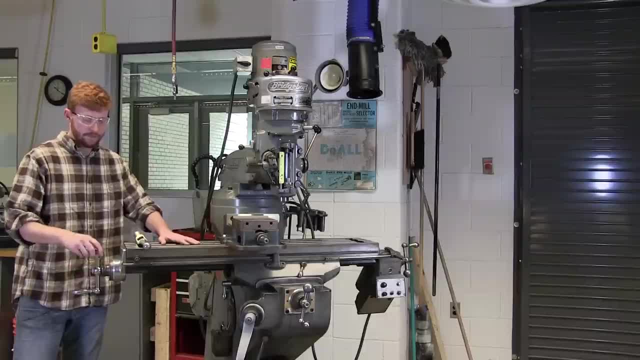 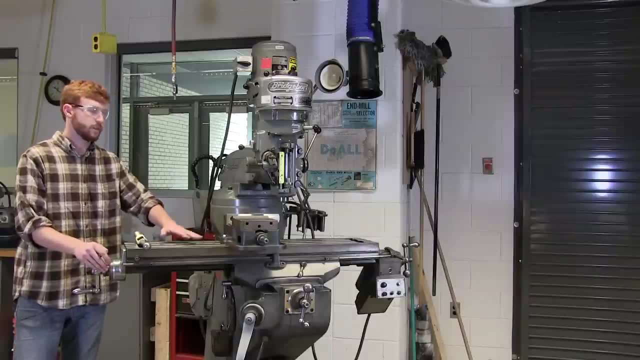 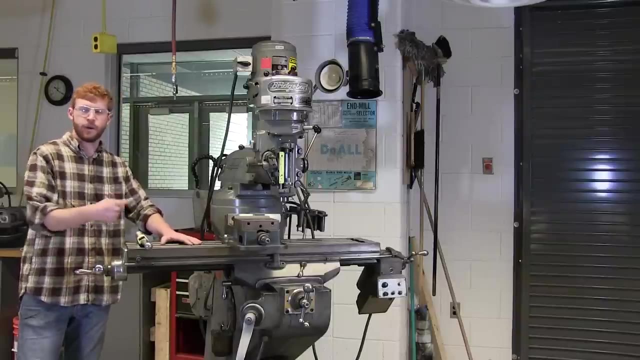 these knobs has a little bit of play in it, Meaning that on this handle there's about 20 thousandths of an inch, that on the knob you can see moving, but it's not physically moving the table. So what that means is, whenever I'm going back to my zero point, I have to come at it. the. 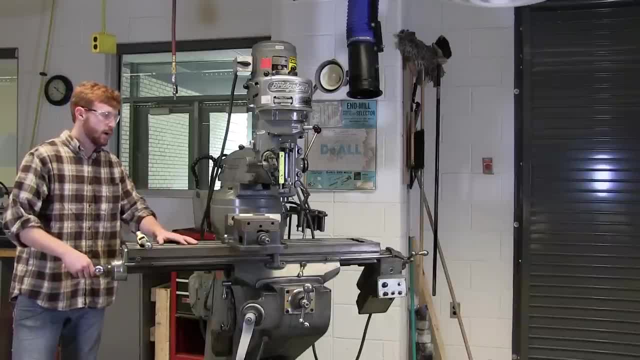 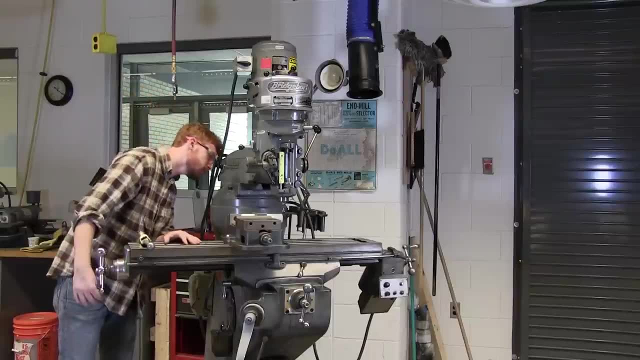 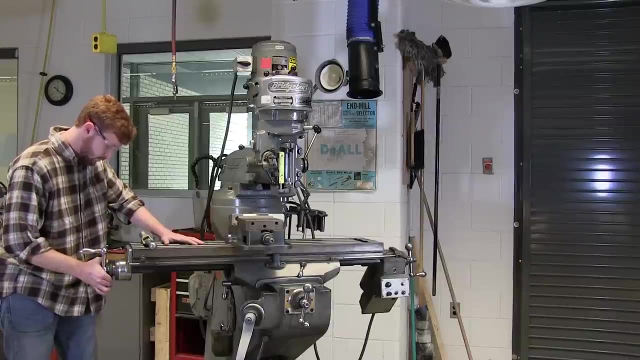 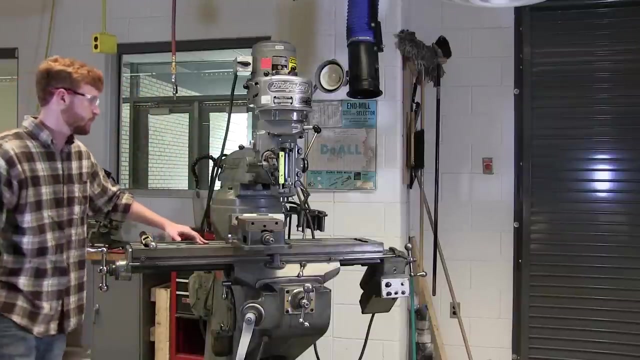 same direction that I zeroed it. Okay, So I move my part up against the edge finder this way. So that's the way I'm going to be finding that zero. So do to my zero. Looks pretty good to me, So that's zeroed. 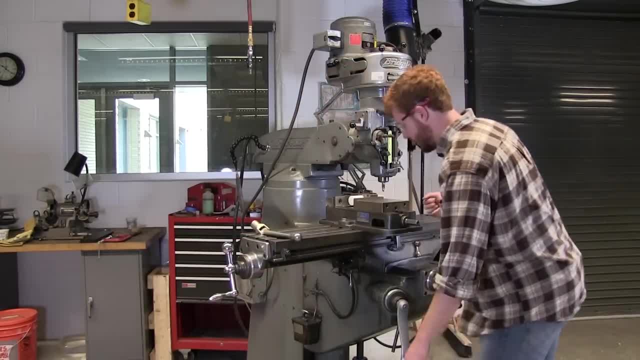 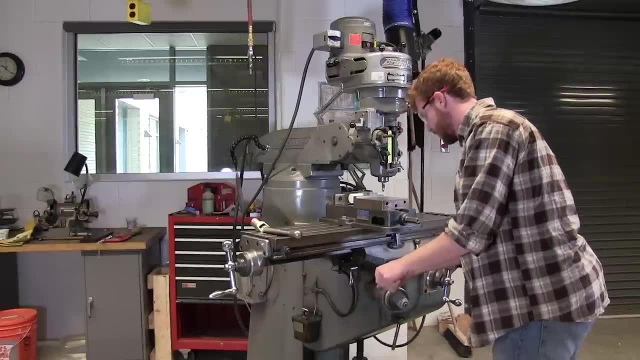 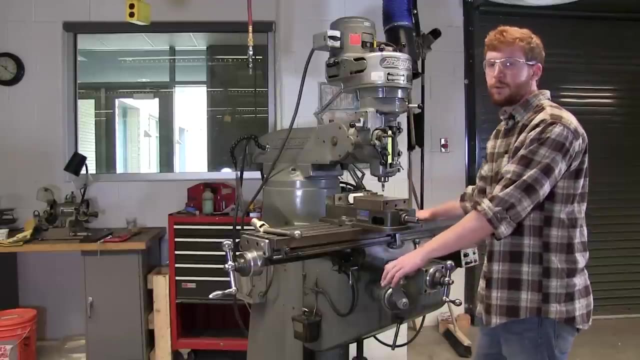 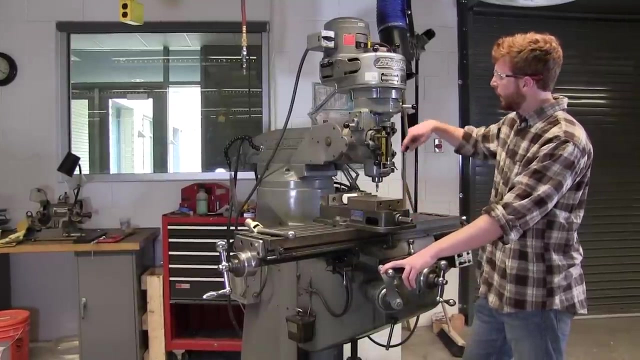 I'll move this a little bit out of the way. Check my Z: Okay, And that looks good to me, So I'm happy with my zeros. I can go ahead and drop my tool down to the depth that I'll be cutting and walk it through. 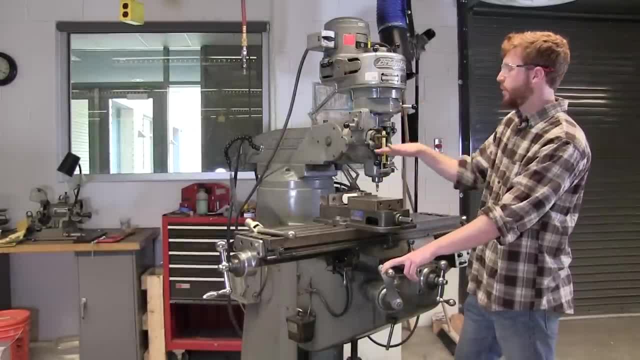 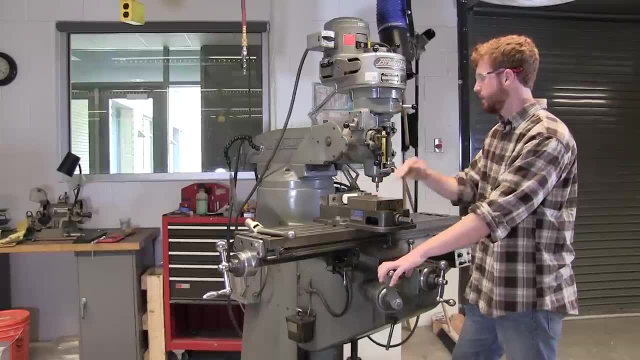 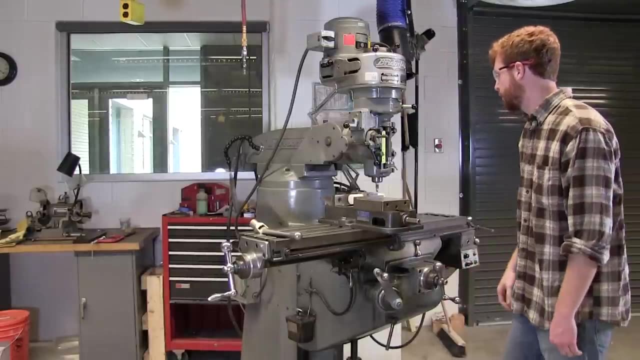 the part, Or I'll actually be bringing the part through the blade, kind of like a lawn mower pattern, to remove all the material. Okay, So that way I have a nice flat base. So I'll move the part out of the way of the tool and from that zero point I'm going to. 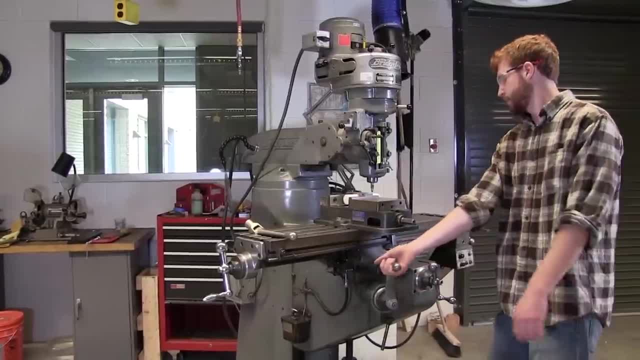 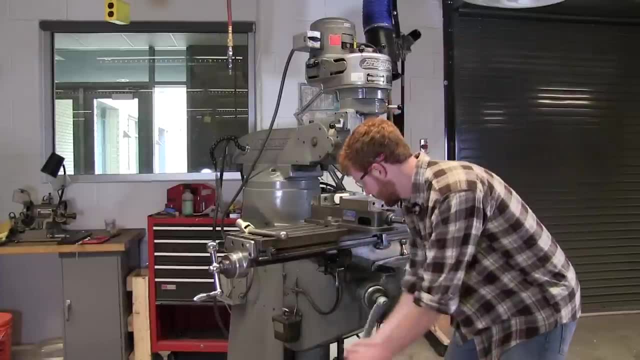 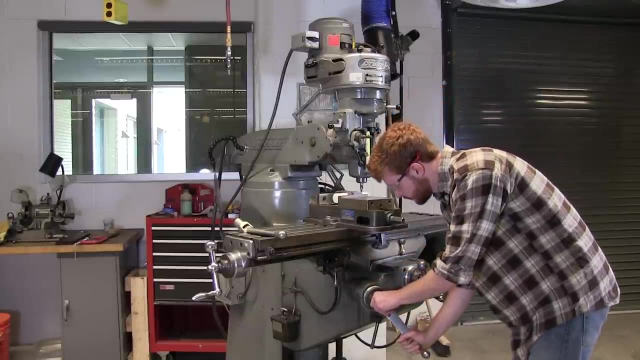 be raising it a quarter of an inch or two hundred and fifty thousandths just to kind of show you guys a cut. One turn on this wheel is a hundred thousandths, so I'm going to be doing two and a half turns. This should end where it reads fifty. 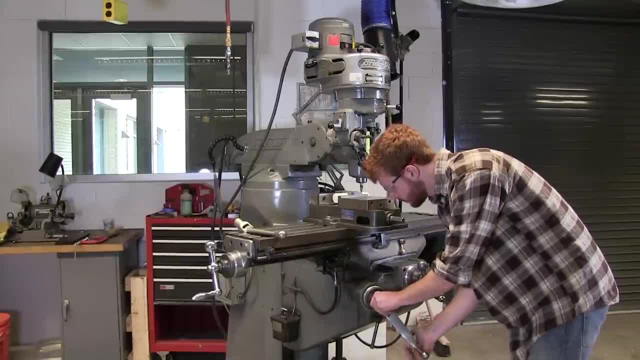 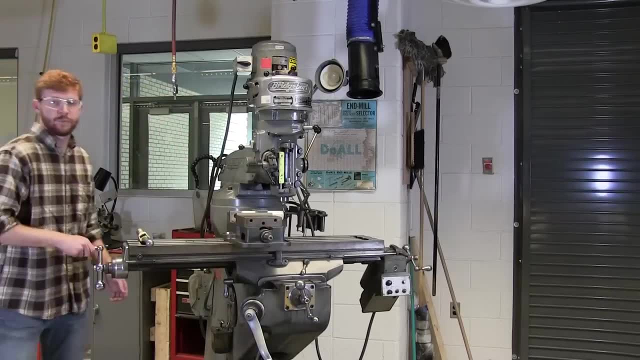 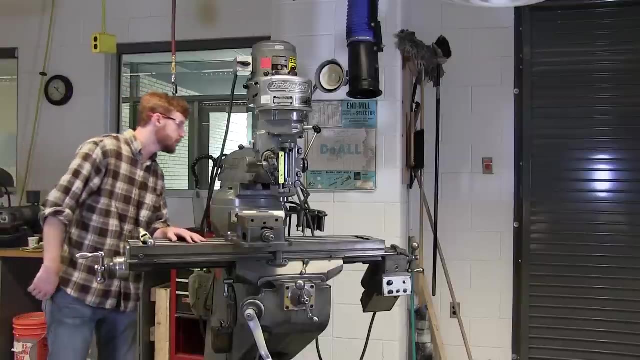 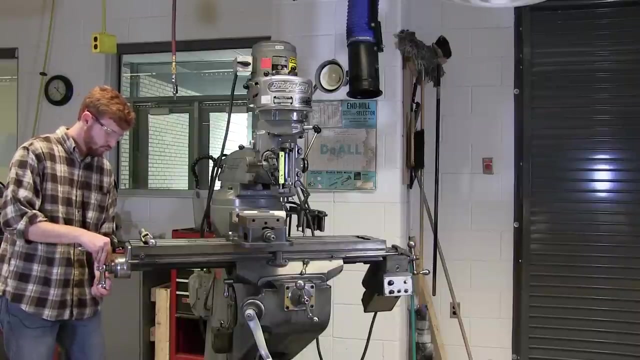 Okay, So that's set. I'll bring this back to my zero, which means I'll actually be cutting into this part with the radius of my bit, which is another quarter of an inch, which is important to know. Okay, So cool, Move it again. 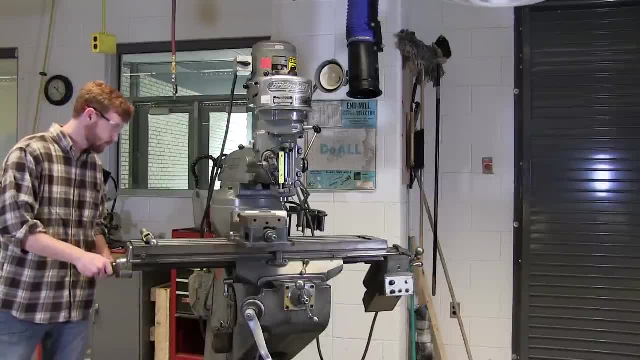 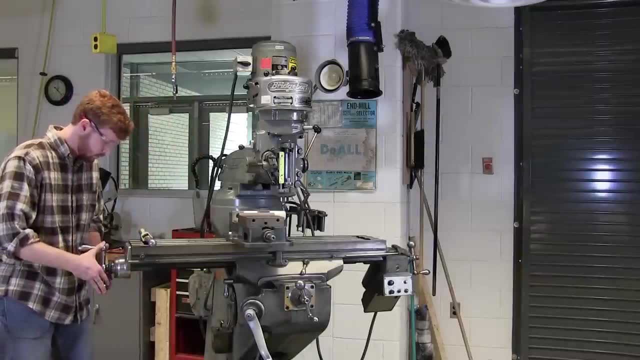 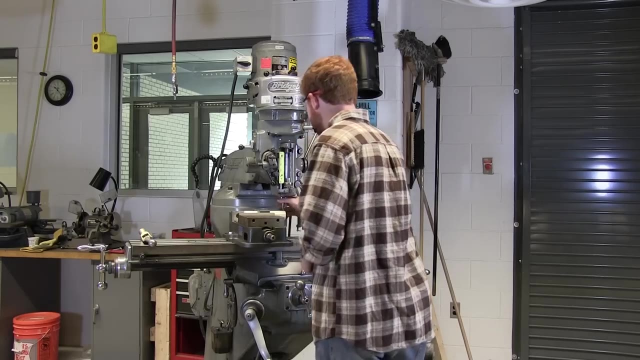 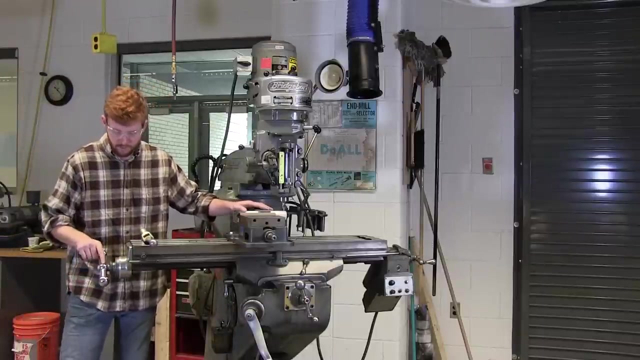 Two hundred thousandths, Two hundred thousandths- Cool. It's kind of confusing sometimes looking at this end and going to your zero. I actually didn't go far enough again, so I'll take it back to my zero And that should be right on. 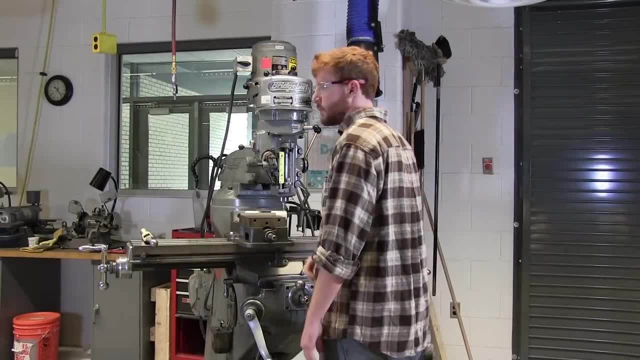 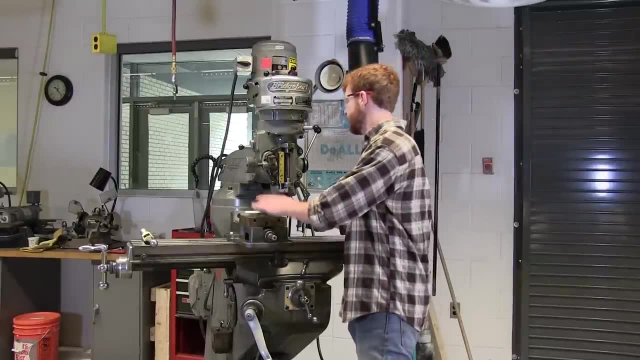 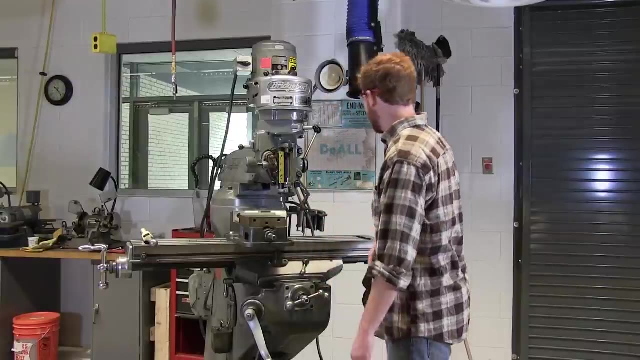 Looks good to me. I can go ahead and turn the machine on forward direction and start making my cut. The way I'm going to do that is, with the machine on I'm going to walk the part into the blade and then, when I'm done with that face, I'll move this another two hundred and fifty thousandths. 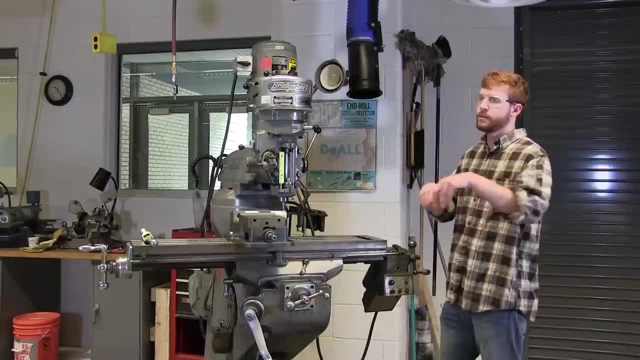 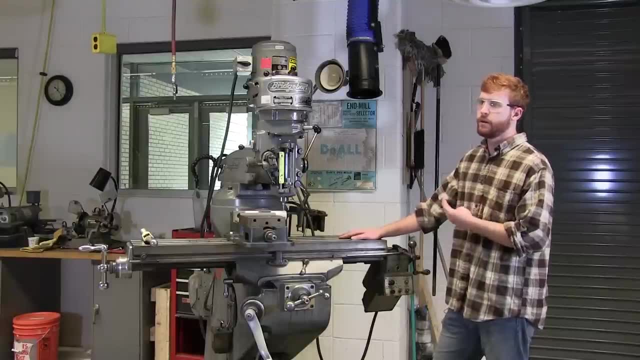 so I'm cutting with like an even depth. So each time it's an even cut And I'll remember where I am And how far I've gone. So I'll make four passes of quarter of an inch each time. ending up with should be almost. 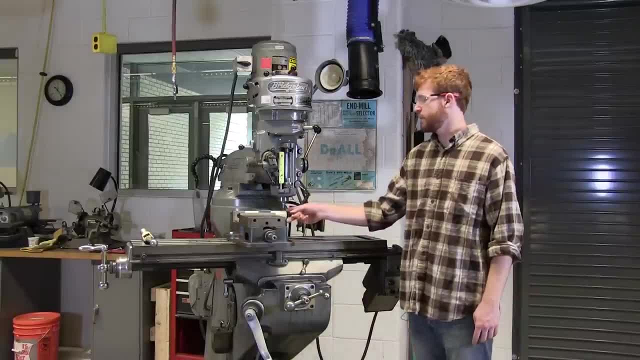 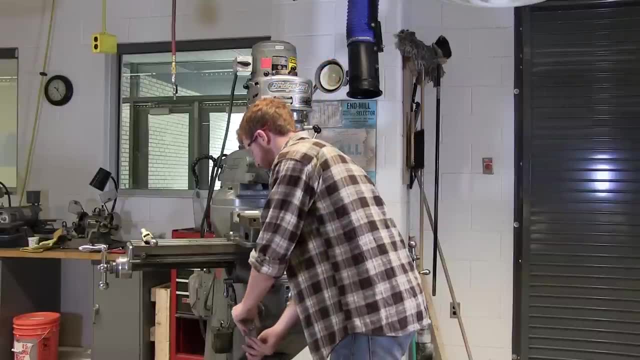 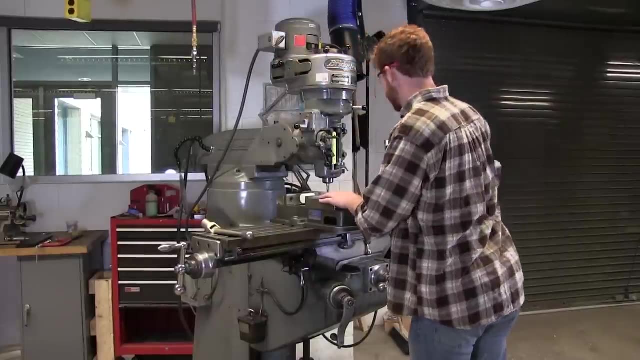 exactly one inch from the very top front face of this to the where I stop at a depth of a quarter of an inch. So I'll go ahead and do that. Take this off, Flip it around, so I don't mess with it And we can go ahead and make our cut. 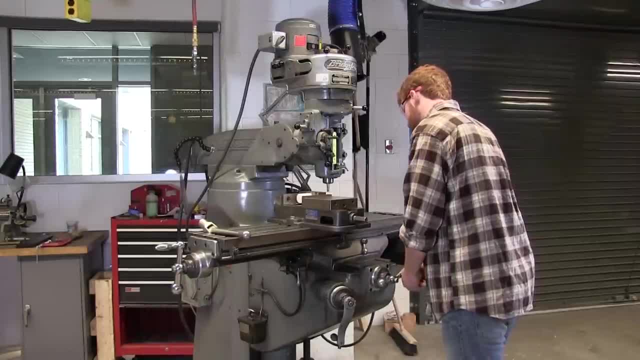 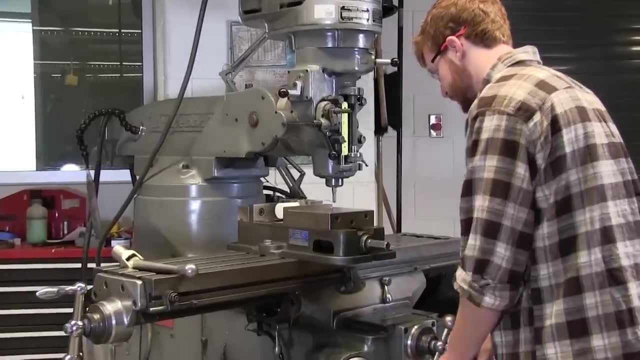 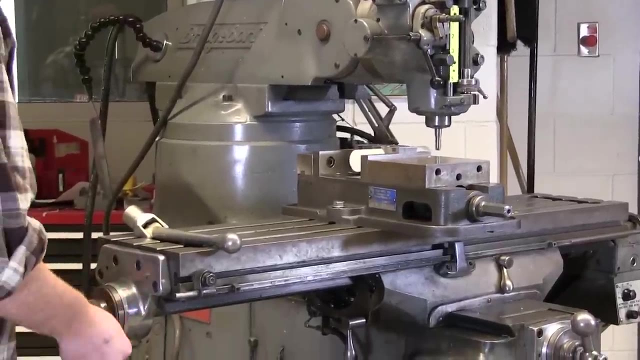 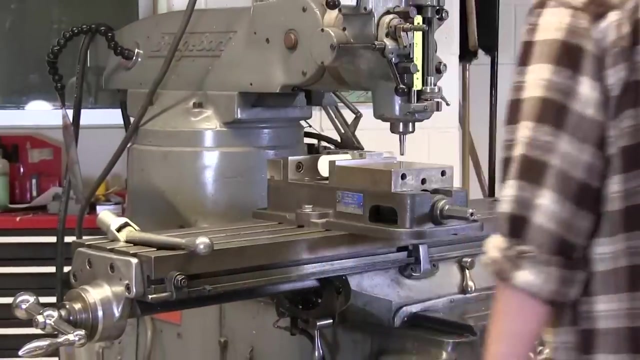 Now I'm going to do the same thing on the other side. I'm going to cut this back in half. So I'm going to go ahead and cut this back in half And I'll go ahead and make four passes And I'll go ahead and cut this back in half.